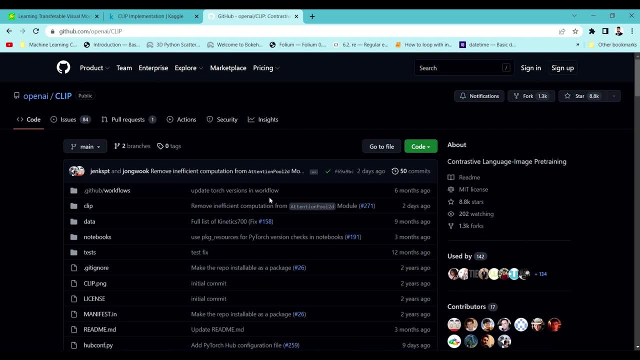 So it's just like a supervised, self-supposed learning that is being taken care of like the BERT model, have been done, trained right. so it's just like a similar training, self-supervised training, without using labeled, without using labeled data, and it is being trained without, uh, without being much interference. 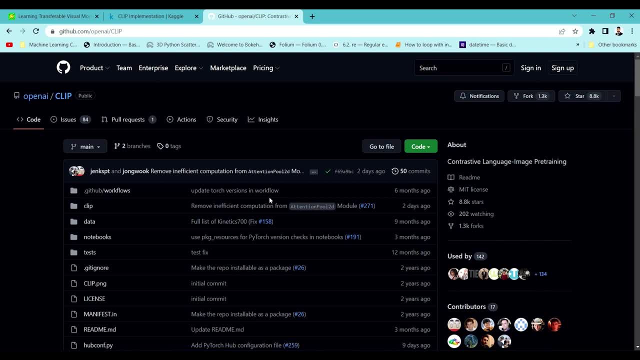 worrying about the labeled data. so it's just a awesome implementation and awesome learning. so we just look upon it and we'll we'll discuss upon the things and if you have any doubts regarding this particular implementation or any of the understanding, you can just mention the things in the comment, where i will try to reply into this, right? so let's now jump jump to. 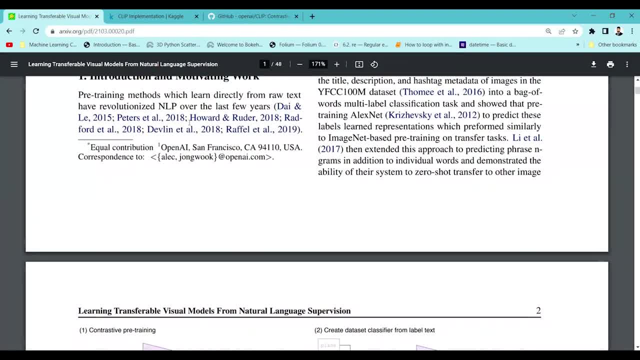 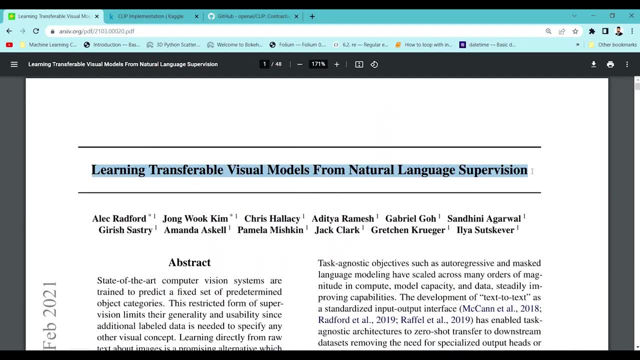 the paper and we'll just discuss the architecture, how it looks like. so, uh, this is just an uh official implementation of a clip or the official discussion where the clip model has been explained, so you can just check out this particular clip or paper and you can go through this clip it has. 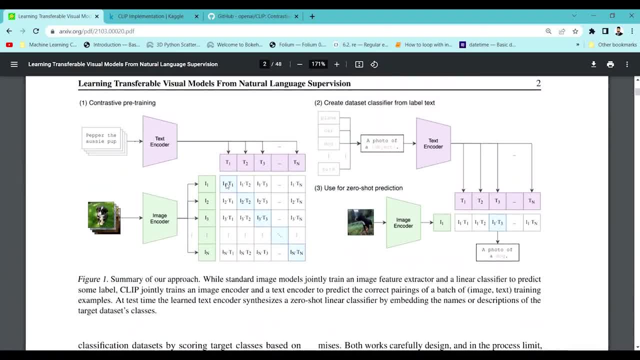 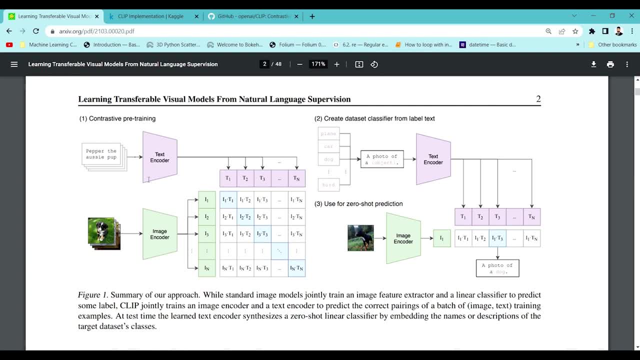 been amazingly explained here how the things has been done, so i will try to explain the things at an at a very high level, uh, but it, it is very, uh, um, it's. it's really very good to uh reach out or read the things in a very 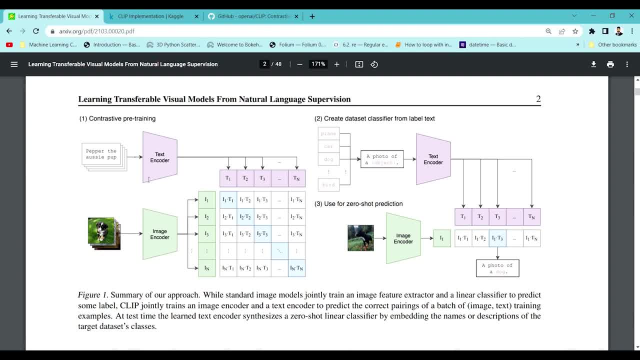 detailed manner. so i will highly recommend you to go through this paper and it will make you understand many other things and it will clear the things so very, very well. so now let's let's move to the architecture part, like how this clip and how this image and text- uh, 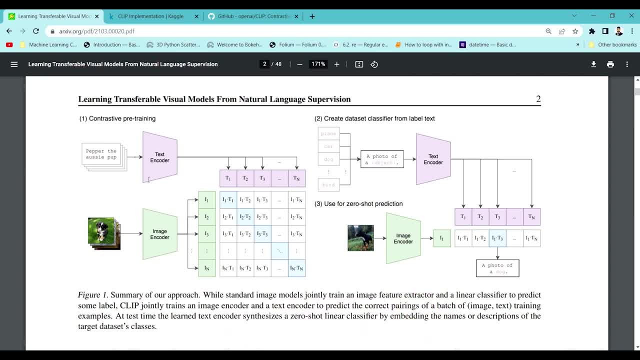 training are being done without using any label, right? so you can see. this is an architecture, right? so what? what is happening here? if you see, uh, you, you go through this particular uh, you can, you can see this. this is a text encoder and here is a image encoder, so text encoder is nothing but. 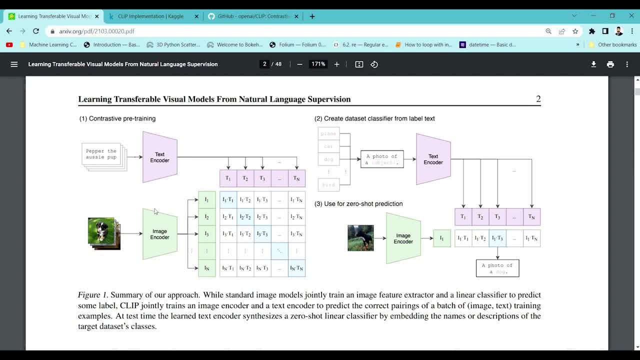 there is some model called bird model or any model like roberta model or any language model. whichever you want to use, you can use it here. so this is just an text encoder where you will input your all the text and it will uh generate an embedding for you. 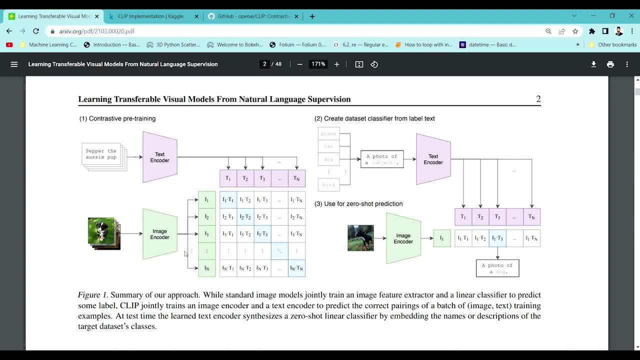 right and similarly, even, uh, you can. you can see, here is an image encoder. there's nothing, but you can use, uh, um, a cnn here here, and you can use visual in, uh, visual transformers, uh, where, where, uh, which which will do a similar kind of thing, where it will take an input as an image and it. 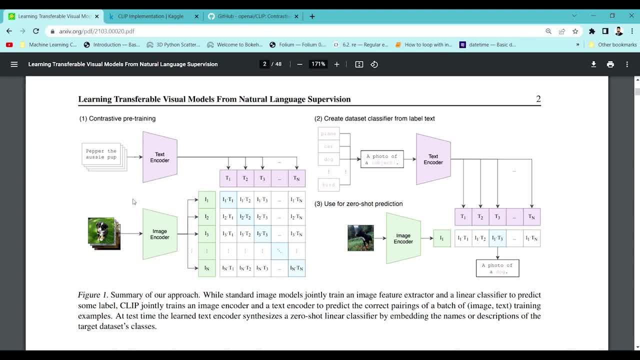 will output as an embedding of particular image. so this is what text and image encoder will do. image encoder is uh. is that? this is what the function of the text and image encoder? so now why we are taking this text encoder and image encoder right? so obviously we cannot pass uh text. 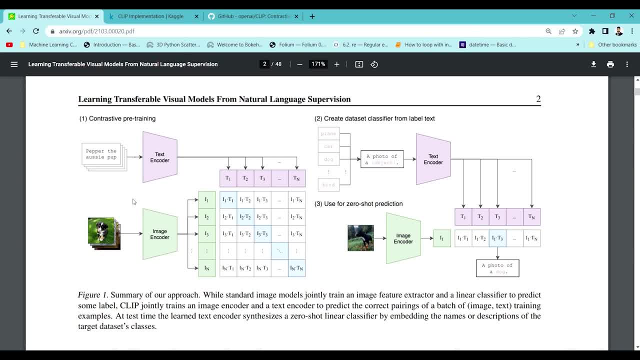 and image as it is, so we have to encode it. so if you use a text encoder as an bird, so it will take up the text and it will encode into the respective embeddings. then it will output something or some, some different dimensions, right? so this is the image encoder and if you use a cnn, you can see that the dimension of this particular bird 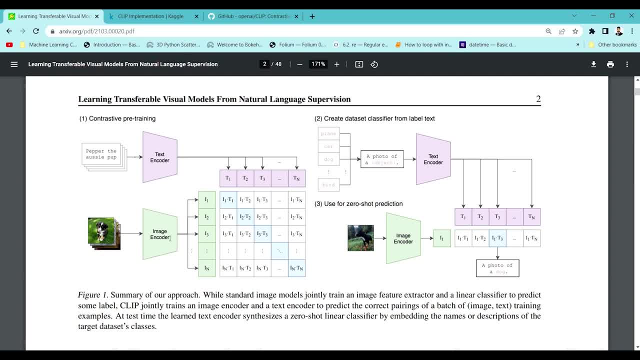 encoder would be like 768, dimension of particular word. and similarly, if you go, if you check out this image encoder and if you're using a cnn network to encode your image, then, uh, their dimension would be different, right? so if you're using a resident 50, their dimension would be 2048 and if you're 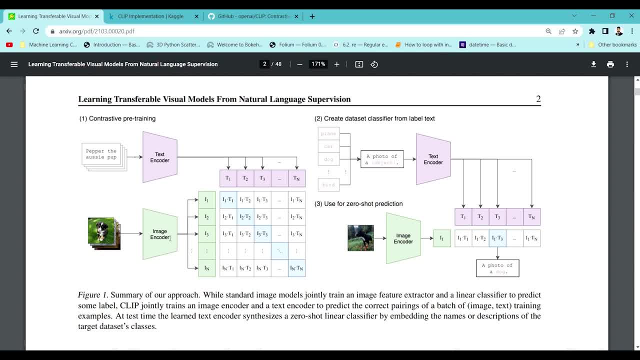 using vid transformers, their dimension could be different, right? so, depending upon the image encoder, Why you would want to use VIT transform and VIT BERT encoder. so what happens here is they use the vertical border and they use uh, vit transformers and resin at 50, whatever model you want to use, or even they used. 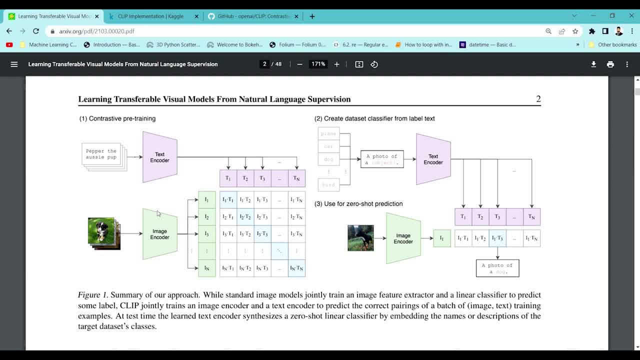 different varieties of model over here. uh, so they have taken up these models. once they have done it, once they have passed the text into the text encoder and once they have passed the image to the imaging code, then the embedding officially completed. the embedding of this particular text encoder will be different and image encoder will be. 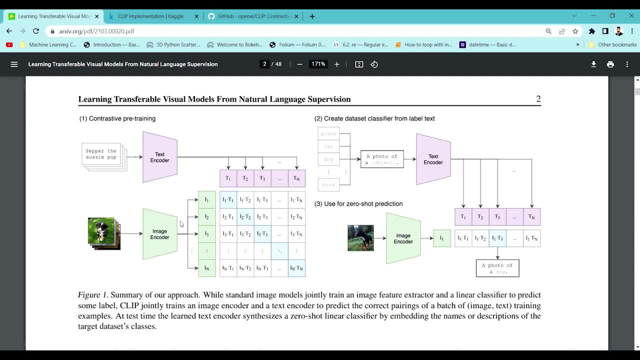 different right. So to bring up that into a similar space or similar embedding space, they have passed this particular output of this text encoder and image encoder into a projection head. So what does that projection head means? is it's just an inner network that will take? 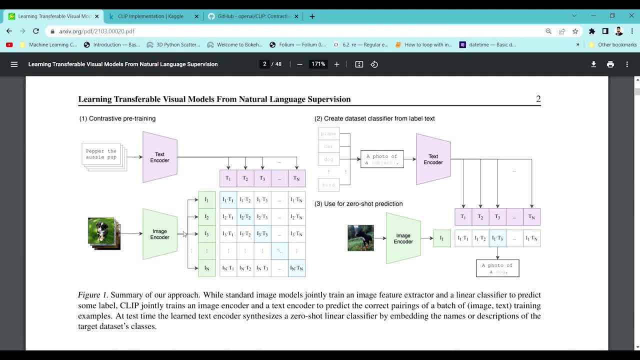 up these embeddings and it will project into the similar dimension space. So what does that mean is that when we talk about the output of this text, encoder so they will pass it to the neural networks or simple ANN networks or multi-layer perceptron, where it will convert into a single dimension network. so let's say 256 dimensions, right? 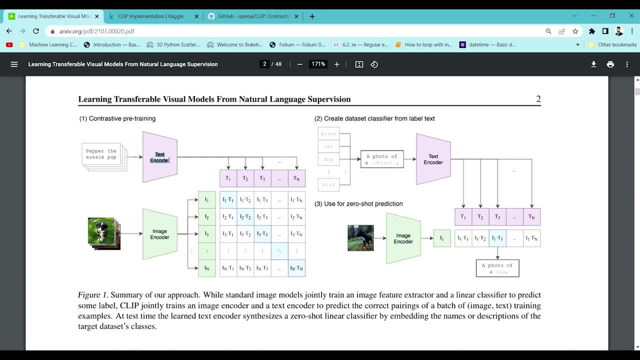 So let's suppose the text encoder has outputted 768 dimensions, so we are compressing it to 256 dimensions. The output of the text encoder: we are compressing it to 256 dimensions by using the ANN network. Similarly, we are using image encoder and we are passing it to the ANN network to compress. 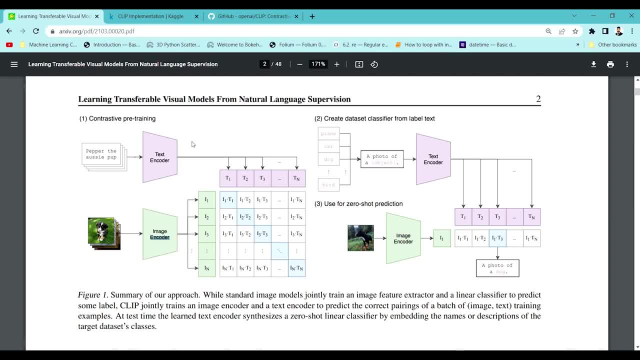 into the 256 dimensions. So then, once we have this- dimensions equal- like the text encoder and the image encoder dimensions are equal- then we can use something called similarity, calculate the similarity between the text and the image, and then that's how we're going to learn the relation between. 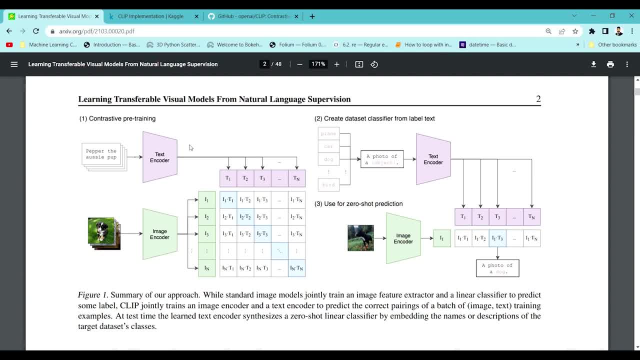 the text and image. So let's go to the next slide. So this was the general philosophy that generally is being done. So now let me explain what happens once we have the dimensions on the similar space, right? So let's suppose we pass an image and we pass in respective caption, or we say the respective 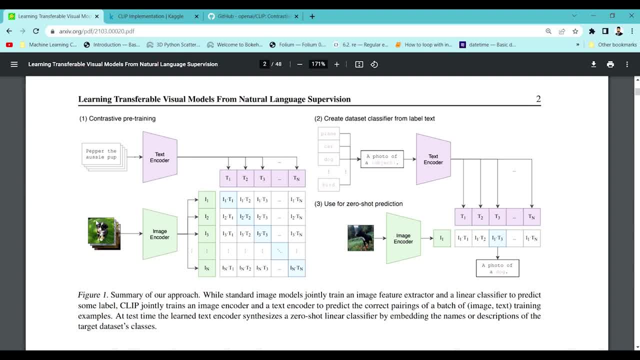 information of that particular image. So we have this dog image and you can see there is a information about that particular image. So they said: paper the Aussie pup. So it's just an information. This particular dog, So its respective image and its respective text, is being passed to this text encoder. 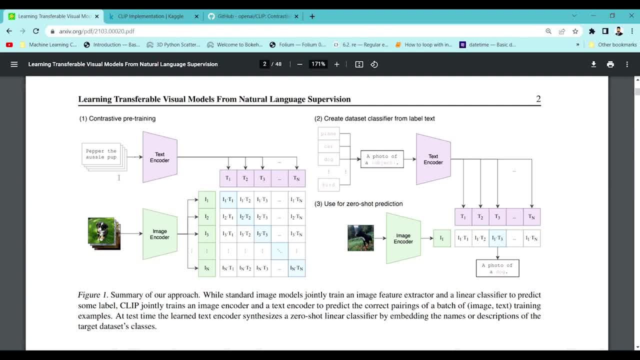 and image encoder. And now we want to learn the similarity, or we want to learn the embeddings of this text and image, right? So how this is going to be done is by calculating a similarity matrix. So if you see here, for each and every image, so this is image 1, image 2, image 3 and so 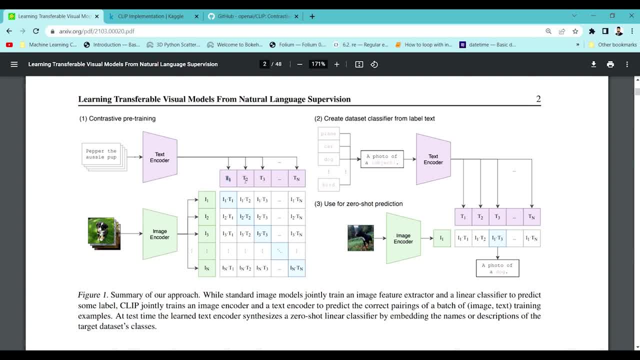 on, and for each image we have text right. So T1, T2, T3, right So. So what we want to associate is, once we have the image embedding and text embedding, we want to calculate the relationship between these two And obviously the first image and the respective text should have highest correlation right. 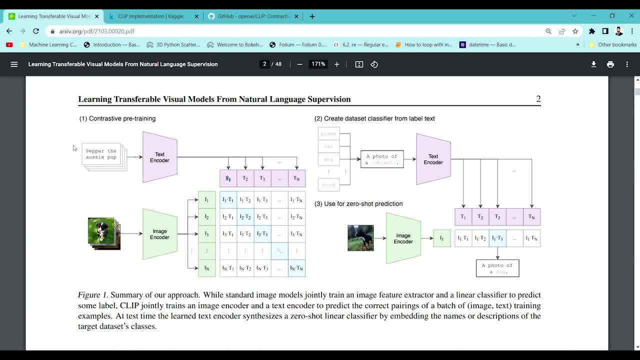 because they are actually correlated, because this particular text is talking about this particular image, right? So this has to be highly correlated with this particular image, right? So that's what that's. what we're trying to learn is just a dot product of this particular image embedding and the text embedding, and we try to learn the correlation between these. 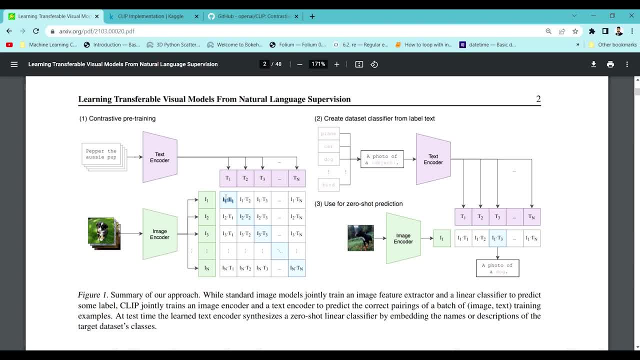 two by using cosine similarity, and that's that's how the loss function is also defined. So we'll go to the loss function, how that particular loss function is being defined and how they're using to get this text and the image closest to each other in the real. 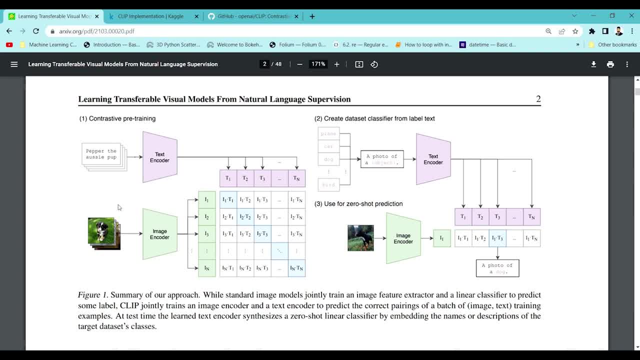 time, Although we know that this is related to this, but model doesn't know right, so we want to make it So for that. these two are related and hence we are going to learn the embeddings and the information from the image as well as text, and we're trying to compress that into a similar 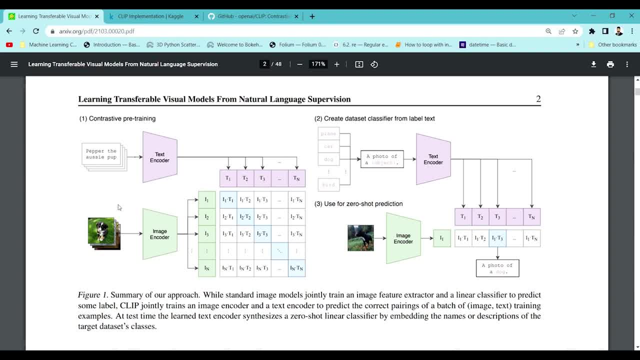 embedding space. So we're trying to compress or find a relationship, or we're trying to relate the text and this respective image into a similar embedding space, and that's how you're going to learn it. Learn the model. That's how the model is going to learn embeddings into a particular space. 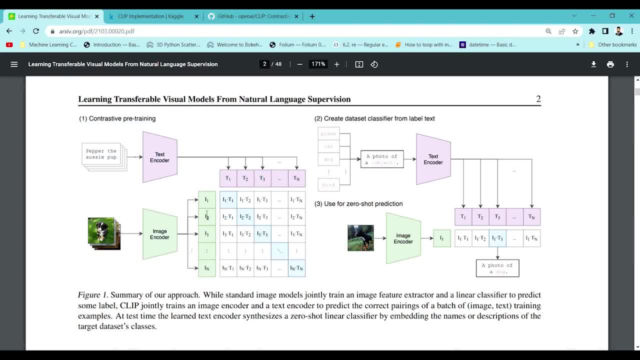 So this is going to be done by using the Different different image. So, if you see, let's go through this first, first line of matrix and we'll go to the second. So what happens is, let's suppose this is the image and its respective text is T1, right? 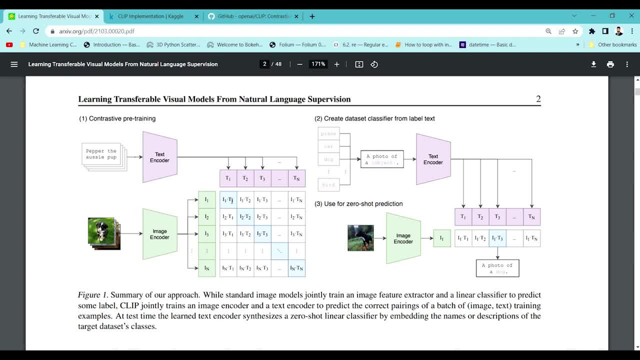 So what it is going to do is it will, it will try to learn the highest correlation, or highest similarity between its image and text and it will decrease the correlation, or we can see the similarity with other text images. Right, So this is the T1 and this is I1.. 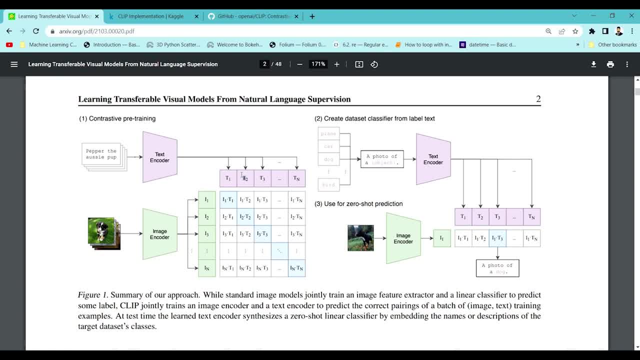 So obviously this dot product should be very high and this T2 is this. this text is different, different image text, right? So the relation between this first image and this second image would be very less. And this and and for the third image. sorry for the third text and the first image, the. 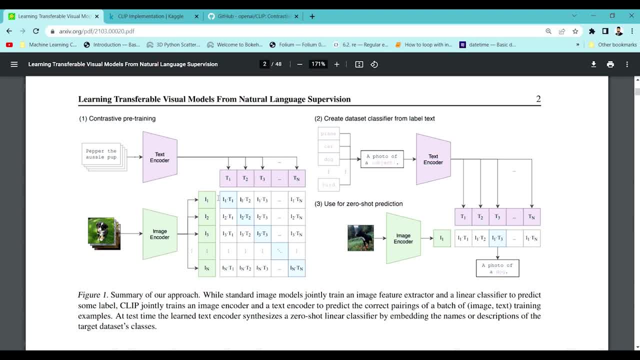 relation should be very less and likewise the others, right. So this is what we want to learn: we want to learn the similarity between the, between the image and its respective text, and we want to decrease the similarity between the first image and the other text image right. 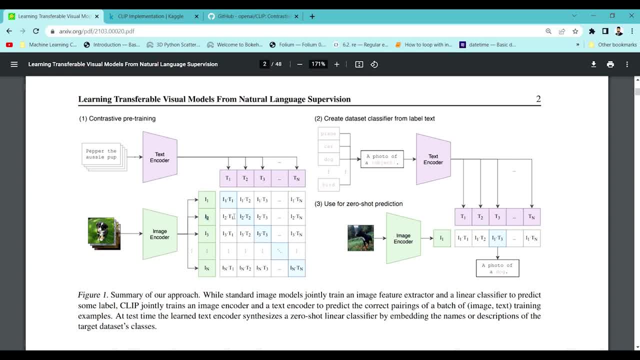 So that's what we want to learn. And similarly, if you go to the image 2, you can see the relation between these two, between the image 2 and the text 1, has to be very low, and image 2 and text 2 has to be very. 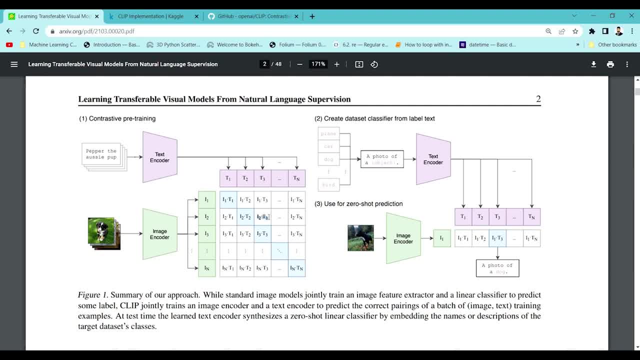 high and similarly, image 2 and text 3 has to be very low. that's how it's going to be learning, So we want to focus on the this, this particular blue part, where it has to learn the closeness about this particular embeddings with respect to the text, and it should also decrease the 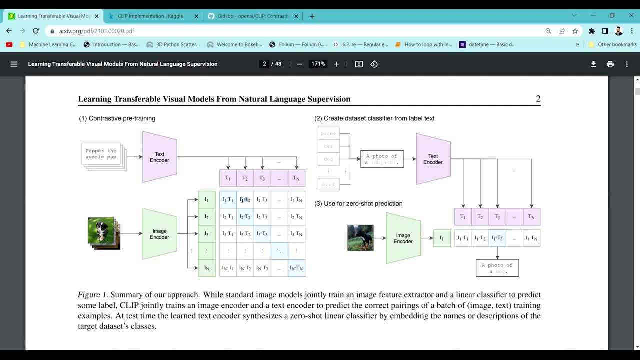 similarity between other text of the images, right? So this is what it is. this is how the model is learning, without any label. So it is itself creating a label for itself by taking this, by considering this as a positive sample. So this is: if image, if image 1 and text 1 are related. 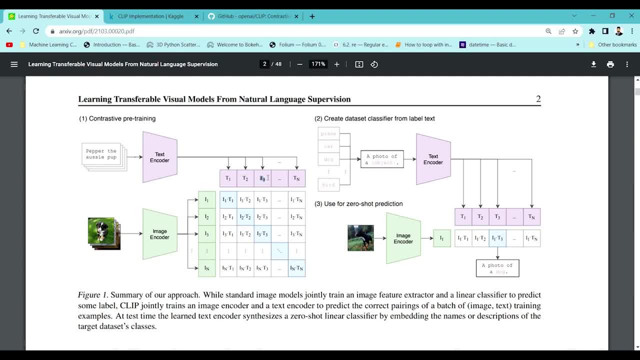 So this is a positive sample for it, and t2 and t3 for the image 1 are the negative samples. So that's how it is creating a label for itself by using this similarity numbers And if you, if you want to dig deeper into the course, 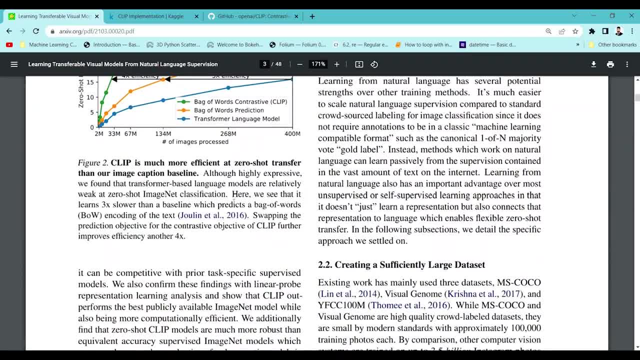 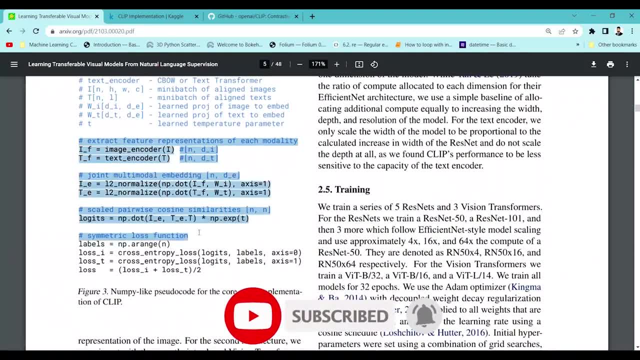 So if you go scroll down into this particular paper, you're going to see how the things have been implemented. So if you go to the loss side, so if you go and see here is the loss implementation, So if you go into this, this particular loss, so if you see this is an image encoder that 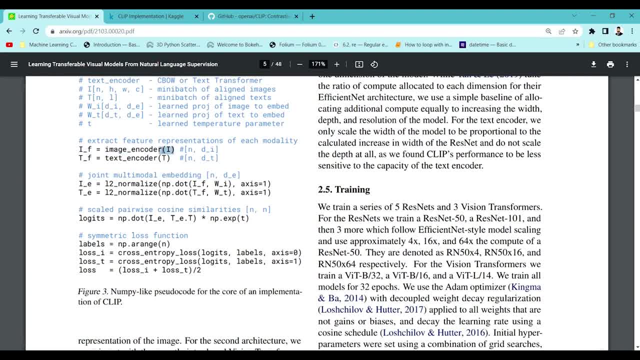 we have talked about in the particular image right at the top. So it takes up this image and pass into the image encoder. it will get the image embeddings. then you pass the respective text of this particular image through a text encoder. it will give you text embeddings. 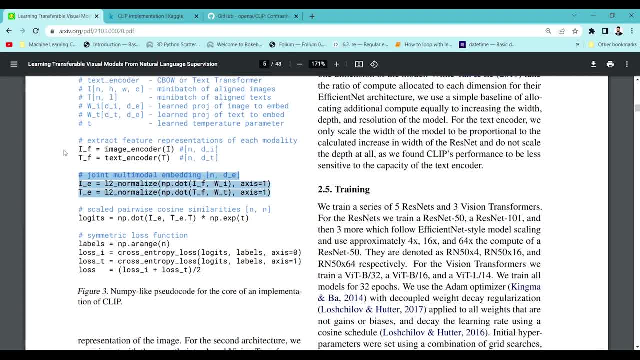 Now what they do is they just normalize this particular embeddings, whatever the embeddings you got from here. Why they do that? because they want to make sure that the distribution is almost equivalent, because text encoder might might give different distribution and image encoder might give different distribution. 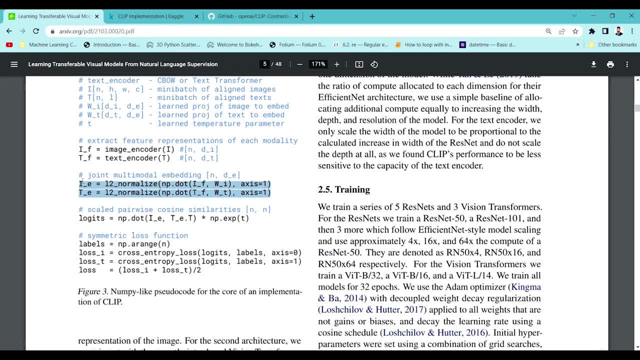 So to make it normalized, so to make it a similar distribution, they are normalizing these two embeddings and now they are calculating a dot product. so you can see it is taking an image and its text and that they are doing a dot product of it. So that's what, that's how they are calculating a dot product. 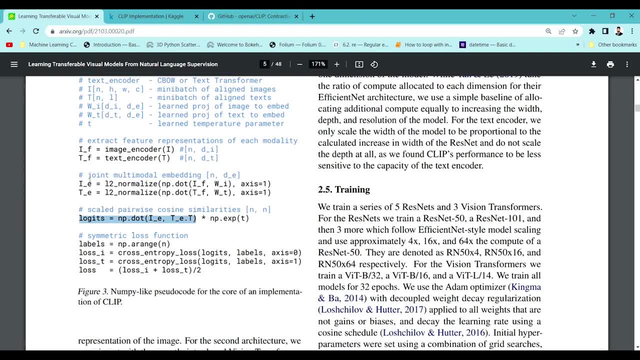 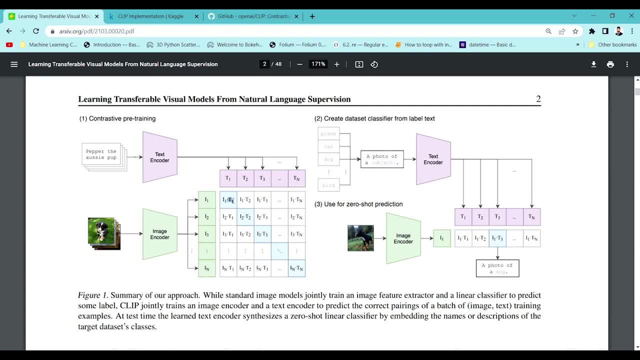 So that's how they are calculating a dot product. And now, once you have this dot product Of the particular image, so if you, if I, have to go to the top of the image, that's what they are calculating here. the dot product you can see right I of image one and text. 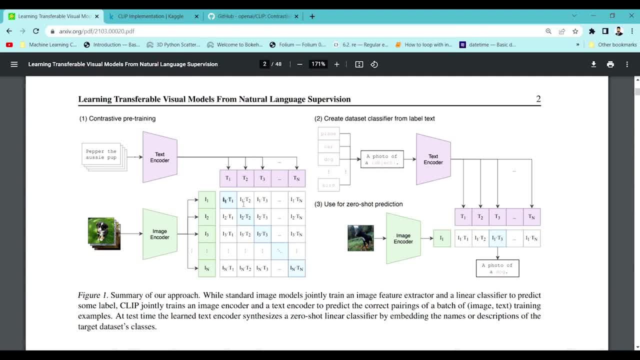 of one. So that's what they are creating. they are calculating the image. that that's what they are calculating: the dot product with its image and its respective other images. So they are calculating the dot product from its text as well as dot product from other. 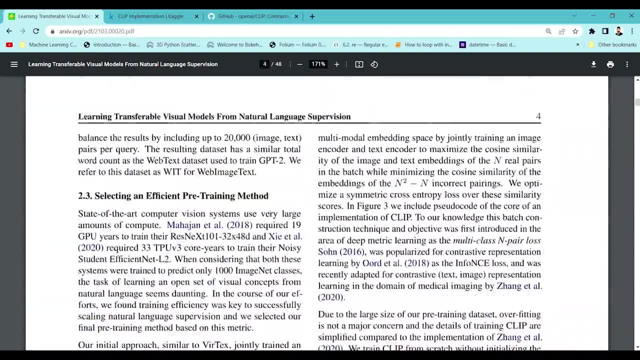 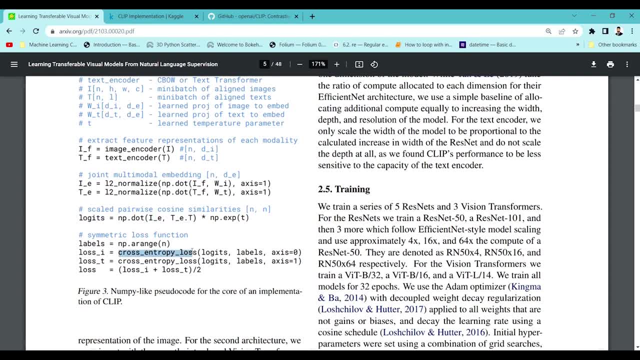 other text also, That's what they are doing here. if I go ahead down, then this is the thing they are doing here. and then they are calculating the cost, entropy loss functions, considering the logitics and the label. So that's, that's a part of a contrastive learning, whatever the dot product they have taken. 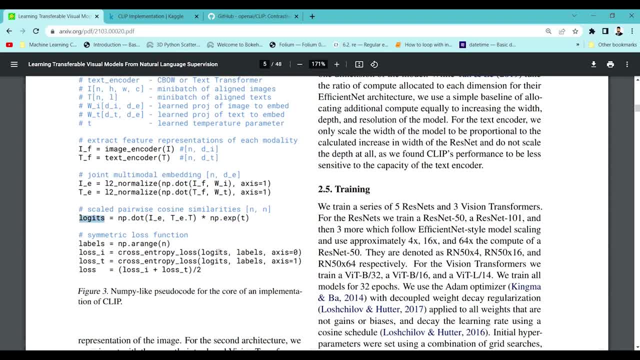 So that becomes a predictive loss, so that becomes a predictive logitics, logits, and then they also take up this labels. So from where this labels are coming up, those labels are nothing but the positive samples and the negative samples, and they're going to create and they're going to generate the 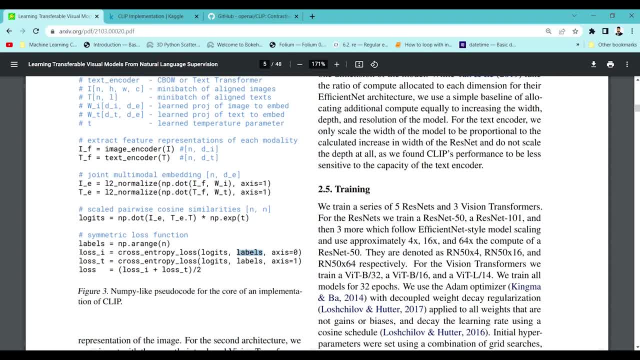 self labels from here. So, and once this image loss and the text loss are being calculated, then they're going to average this loss to calculate the generalized loss, right? So that's how they're going to learn the embeddings from here, if you want to like, if this has. 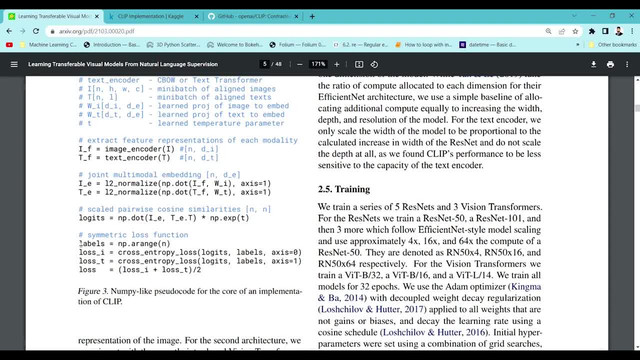 to be done using the code Right, So it's very easy. It becomes very clear when you do the coding, but I will explain this once more when we go to the code Right, So that becomes very clear how we are, how we are actually trying to calculate the contrastive. 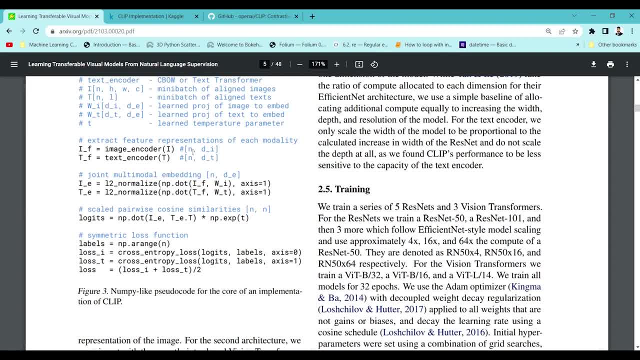 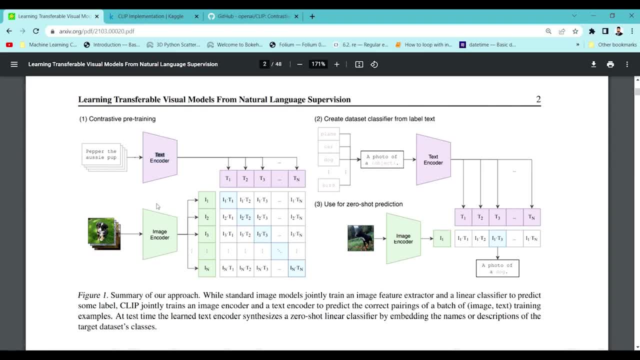 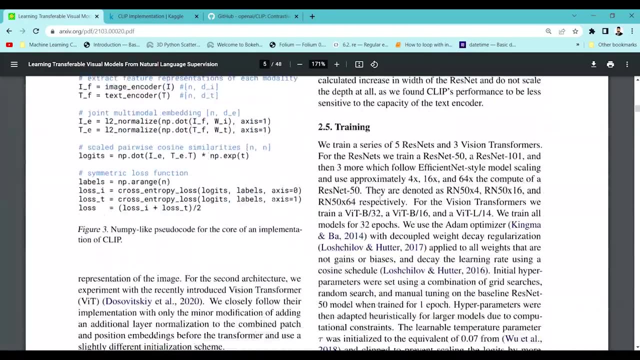 loss. So, if I have to explain more on this, what are the encoders they have used? So they have used, like they are using, obviously, BERT and the visual transformers to calculate the encoding. So if I go to down, So if I go to down and you can see they have tried many of the encoders for the image like 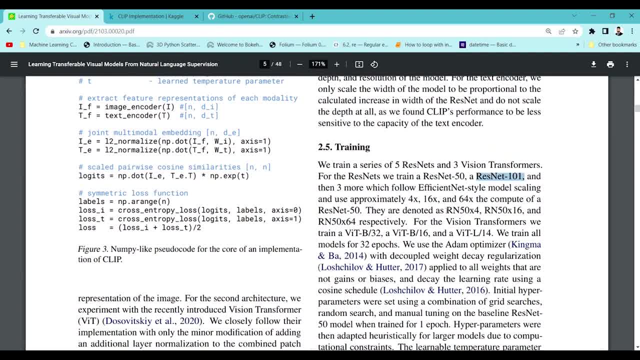 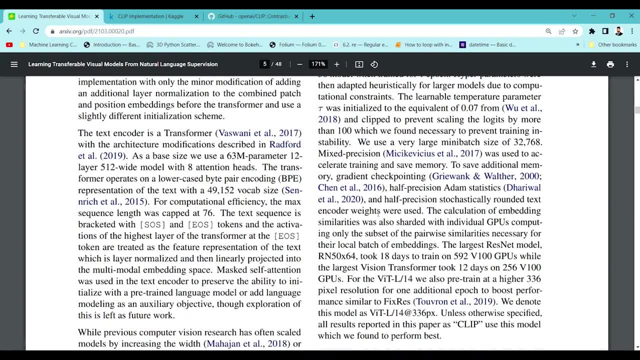 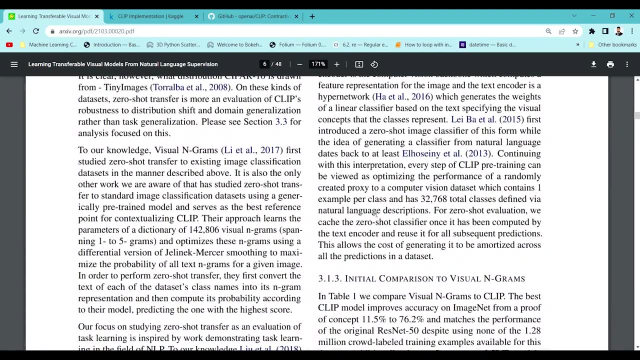 Resonate 50,. Resonate 101. they have also tried VIT 32 with VIT P16 and VIT L614.. So they have tried a lot of a lot of text encoders and image encoders to encode things and learn the embeddings by its own by calculating the similarity between each and every image. 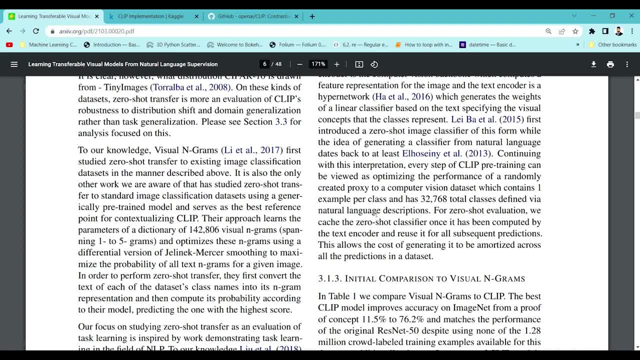 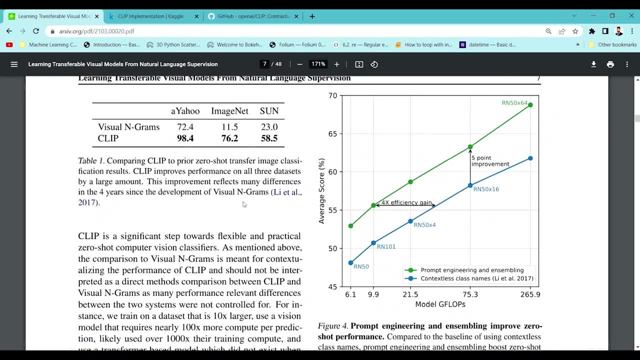 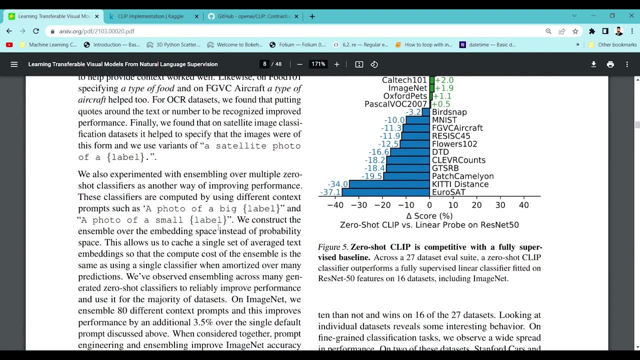 and text pair And also and also calculating the contrastive loss by using that correlation, right, by using that co-similarity. So that's just, that's an high level view of particular implementation of a clip, like not implementation, just understanding of paper. Meanwhile you can go through this paper and you can understand more of the importance. 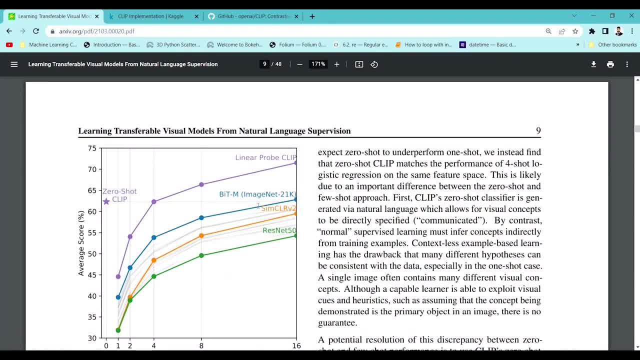 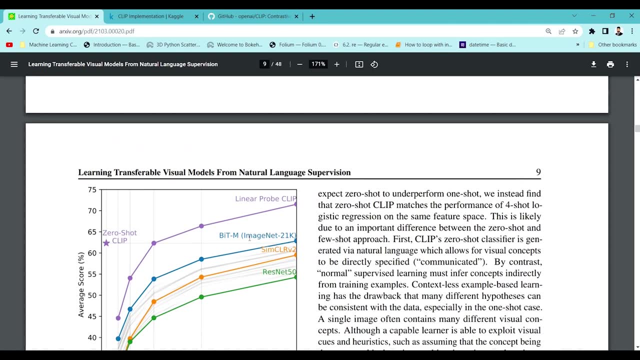 where it went good. So there are other papers as well, like SyncCLR and BITM. These are nothing but image-to-image contrastive loss learning, so you can go through this paper as well. So these are the upgradations to the previous papers that has been done now. previously they 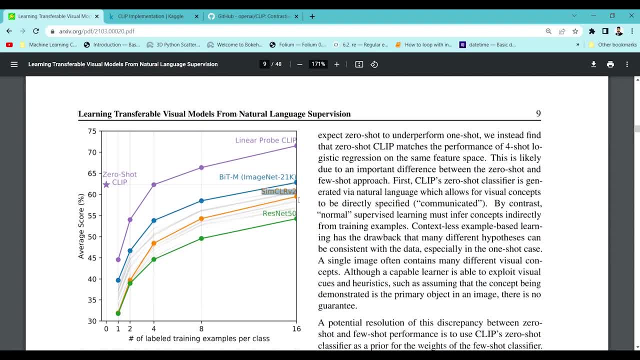 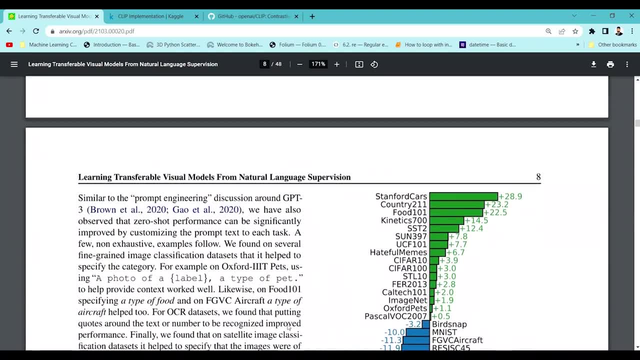 were doing just image-to-image similarity calculation, which was based on the contrastive loss, which I have discussed just now. Now they are doing the same thing with respect to the image and text relationship. So if you go through this particular paper, you understand a lot of things and what the 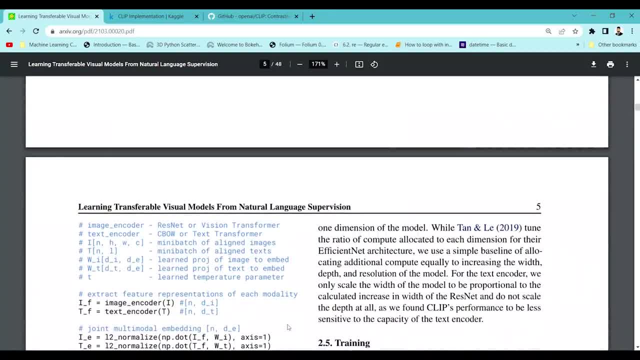 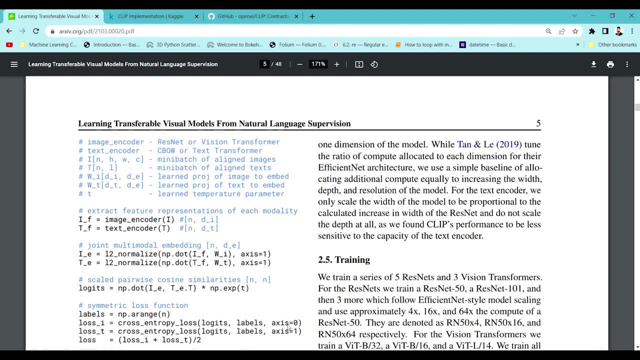 model will output. The model will output the learned embeddings Of an image and the text. So if your objective is to calculate or to get the nice embeddings of an image as well as text by using a single model, and that too they are too related to each other- then this: 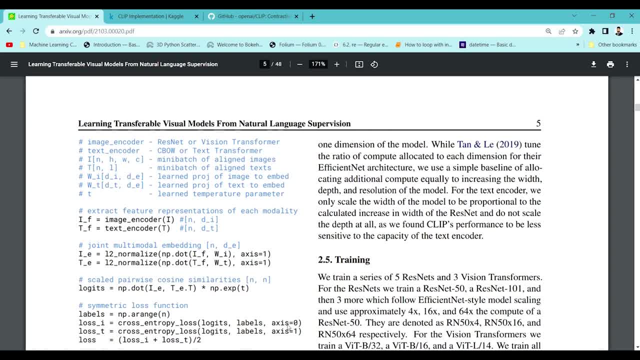 is a model for you. So what you can do is you can just train an image and a text. if you have an image and a text of a respective image, then you can train a model like a clip model, and you can get the embeddings of an image and text. 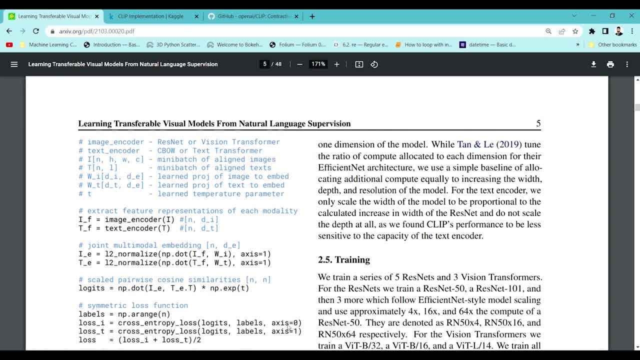 And then you can use it As a classifier to classify it on anything, if you want to classify it on a particular category, and you can do it for zero-shot classification. you can do it for like. you can take embeddings of this particular image and text that are related to each other, and you can do n number. 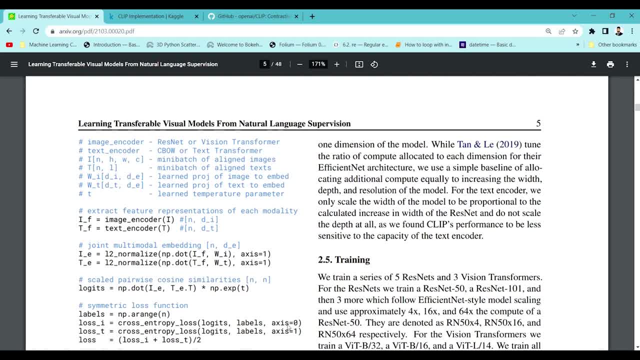 of things with that particular embeddings, right? So that's like an use cases that you can develop with this particular learned embeddings, and that, too, you don't have to have a label data. So that's it. It will create the data or label that the target labels on its own by taking itself. 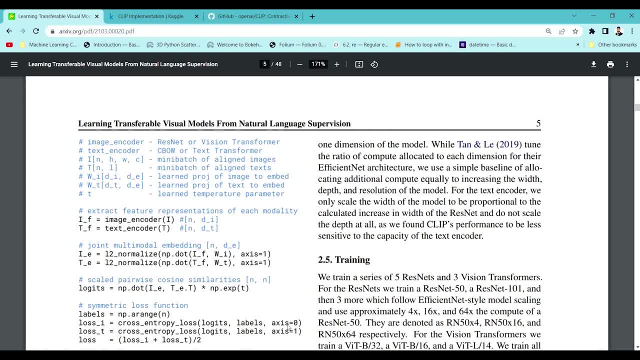 as in its text, by. let's suppose an image and text have its image and text has its relation right, So that becomes a positive sample and other text of a particular image becomes a negative sample. So that's how it creates a target and label for it to start understanding and decrease. 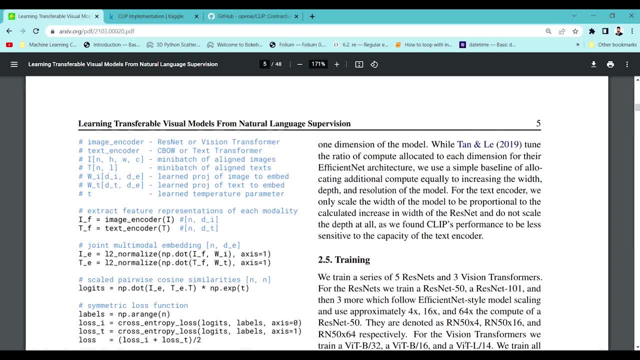 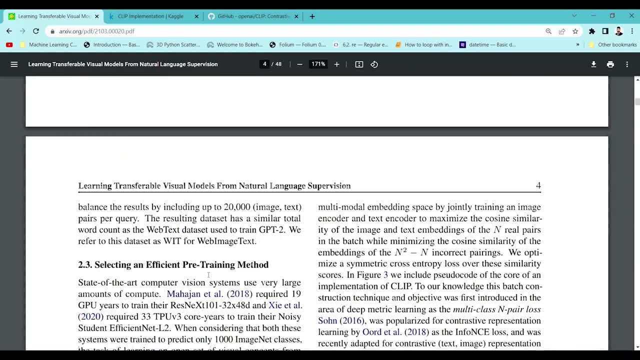 the loss. So that's how we do it. Now let me just go through the implementation of it and things will become very clear. So this was just an overview understanding. So I found a very good implementation of the Kaggle with the Crip implementation. 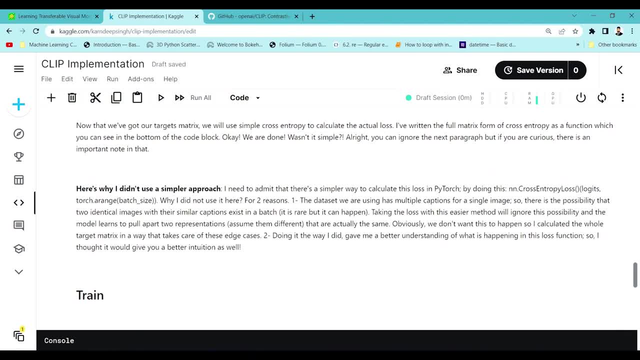 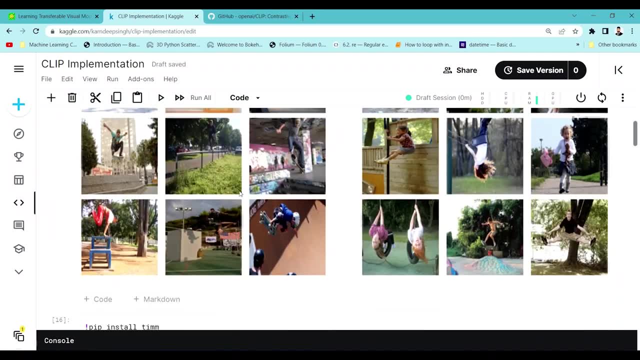 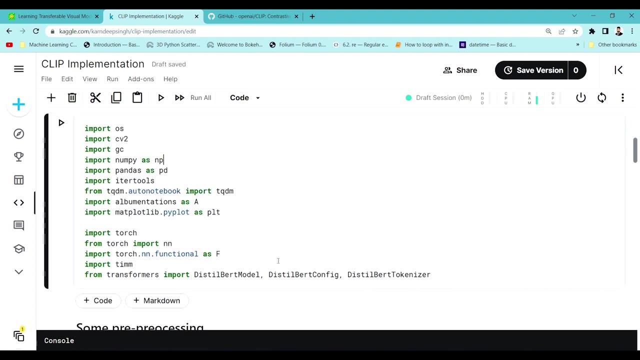 So I'm just walking through it and we'll just try to see how the things work right. So let me go through this particular implementation, what I can see on the Kaggle. I found this very useful. So these are just 10 simple imports. you can see they're using Distilbird and Distilbird. 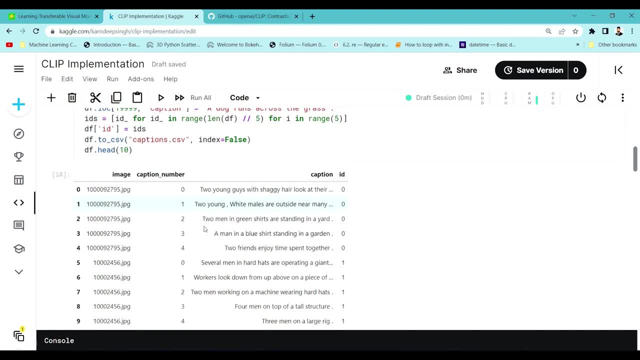 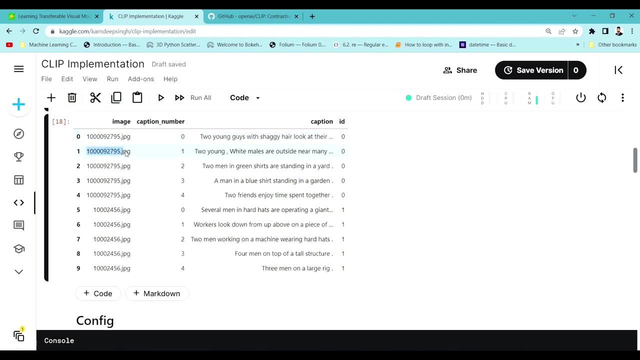 Organizer from Transformers. So this is data. if you see this data, they have this image, the image and its respective caption. So if you see there are multiple just for this particular same image, we have multiple text associated with it, right, And similarly, we have different images and their text associated with it. 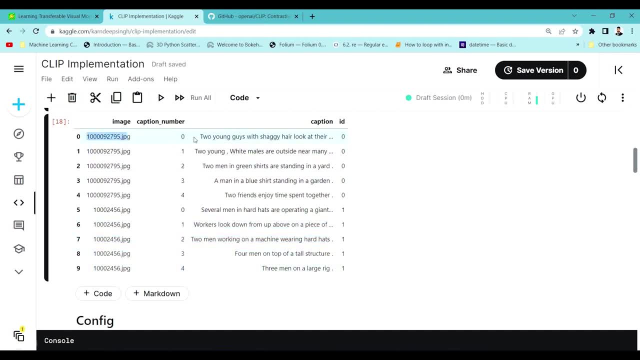 So what you want to do is you want to learn this relationship between this image and the image, and this is all text related to this particular image. So that's what the embedding you want to create. So it will learn the embeddings of this image and this text together, and they also will. 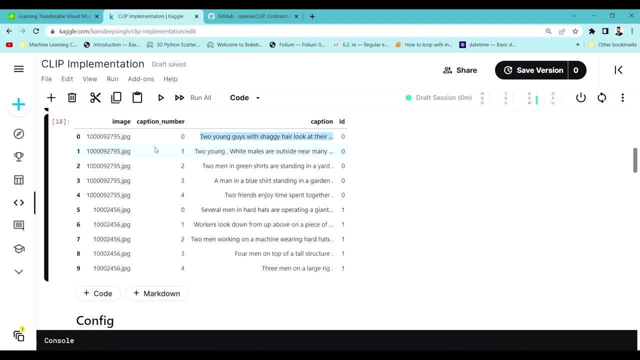 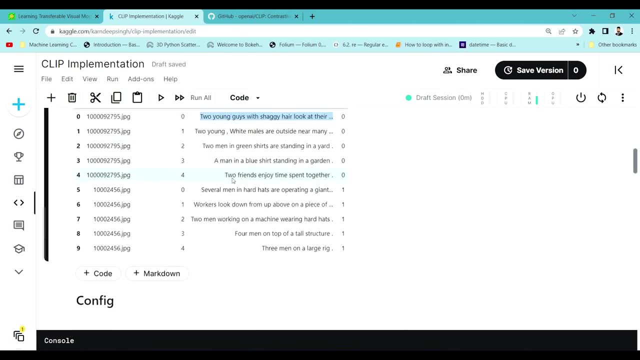 learn the association between these two- image and text- right. So that's the importance of this particular contrastive learning clip paper, and we'll see how it works. So what we're going to do is we're going to take up this images and its text and we'll 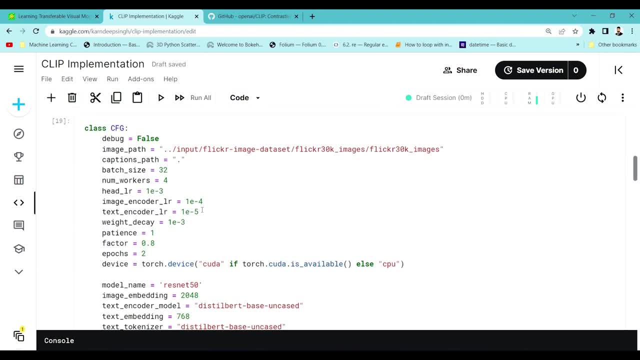 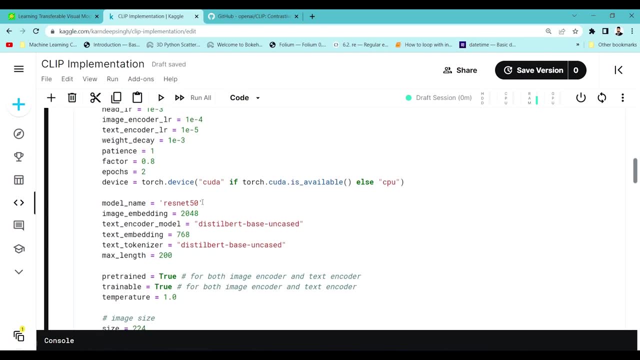 try to encode it. So these are the configuration files. So what we're trying to do is here is we're going to take. we are just trying to associate the different parameters of a model, like if you want to use VIT, Resonant 50 or Distilbert. 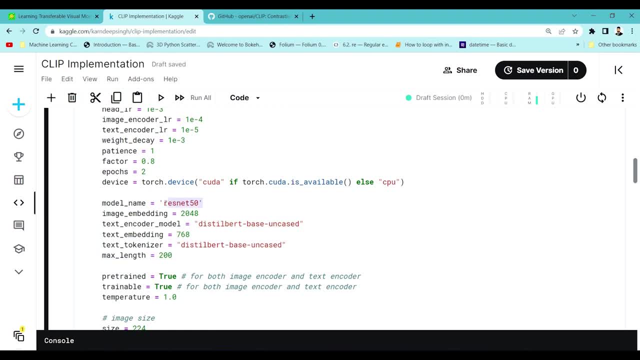 So these are the configuration files that they have mentioned, So you can use any of the any of these things, like VIT or Resnet or any of the like Google Visions models, any of the models you can use for the image encoding, and you can use BERT. 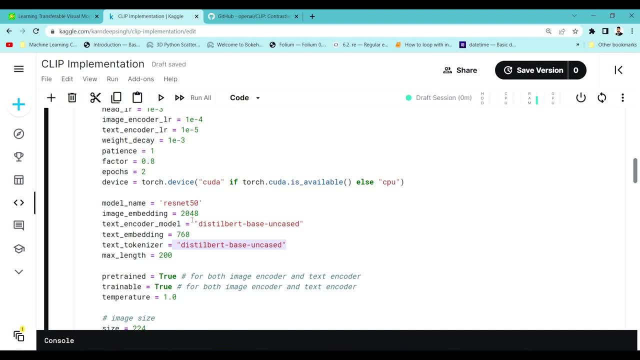 model or Distilbert model or any of the text encoder models. you can specify the models here. it will start the loading and it will do it for you. So right now, as an implementation, what has been done here is they're using Resonant 50. 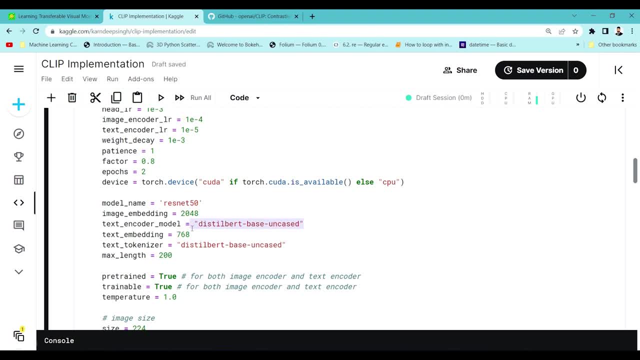 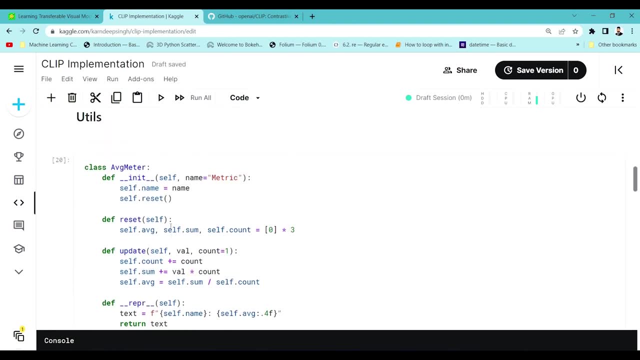 for image encoder and they're using Distilbert for text encoding, right, So they're using these two models and now they're using. now the metric has been also being calculated, So you can just go through this metric and now just this part is for preparing the data. 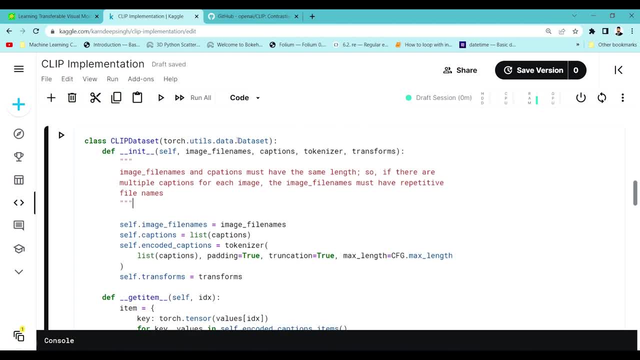 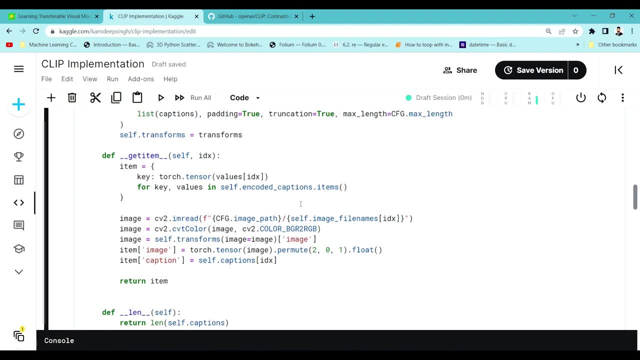 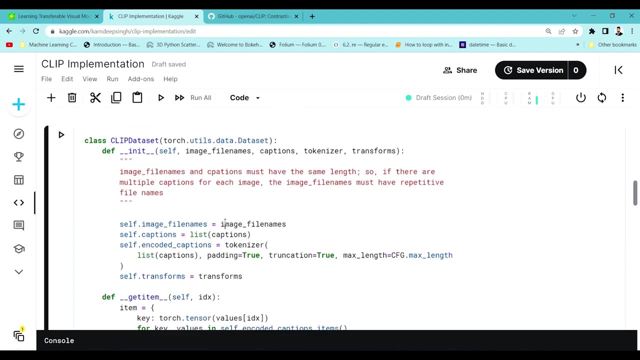 set, like by using Torch data set. So to prepare the data set, They're using Torchutil data set to prepare that. this class you can just go through. it's very simple. It's just not take much time to do it. So what ultimately is being done is they're taking up this file names. 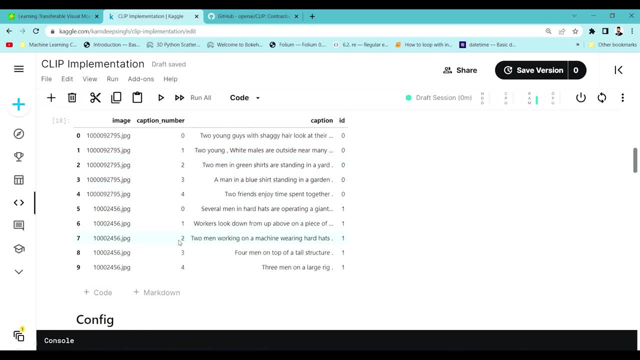 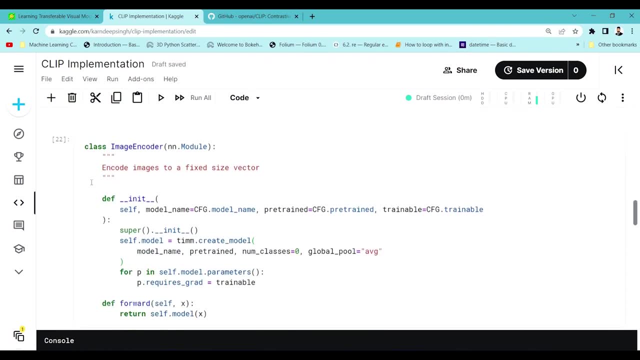 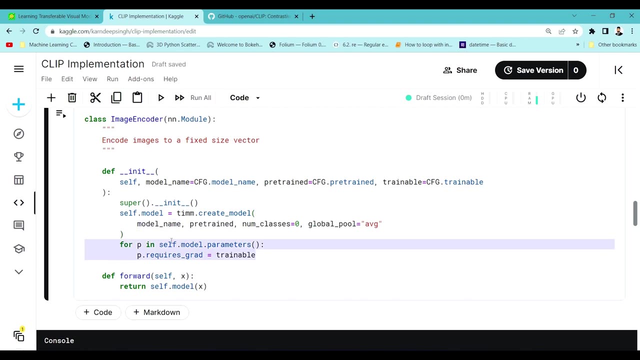 What are the file names? you're provided right image names and this respective text and converting it to the PyTorch data loader. That's what they are doing it here. and this is an image encoder part where you we are loading the Resonant 50 and you're taking up their head of the model. 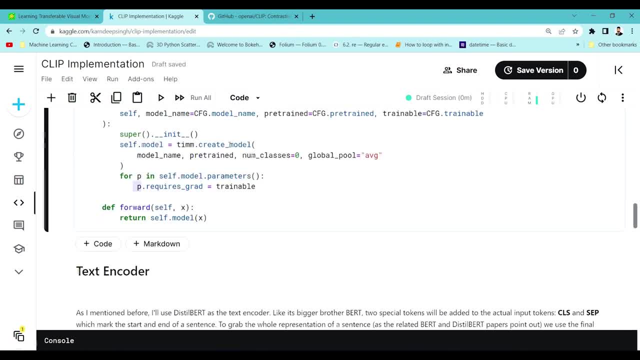 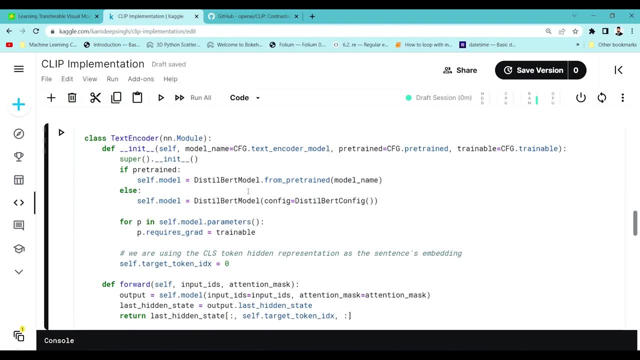 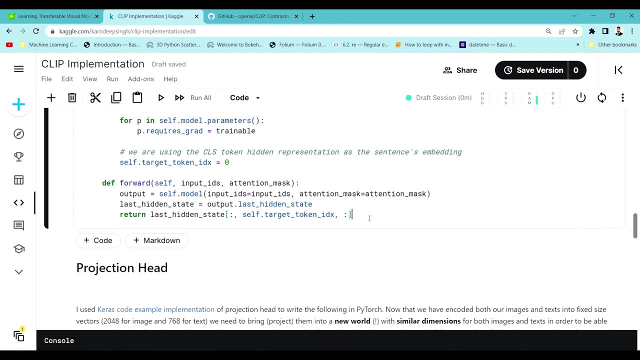 That's what they are doing it here. So it will. if you pass this particular image into this particular model, it will encode the image. Similarly, they are defining the text encoder, they're taking a Distilbert and and it will the freezing of the layers, of the previous previous layer, and they're taking the output. 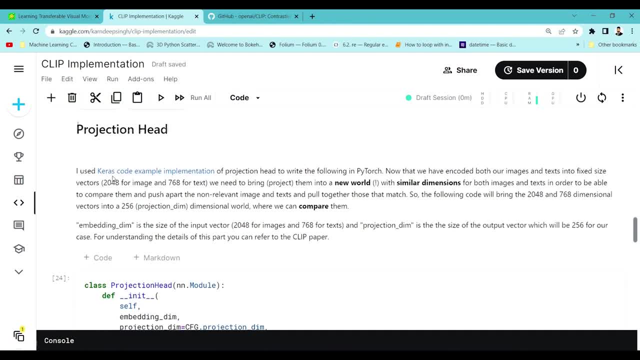 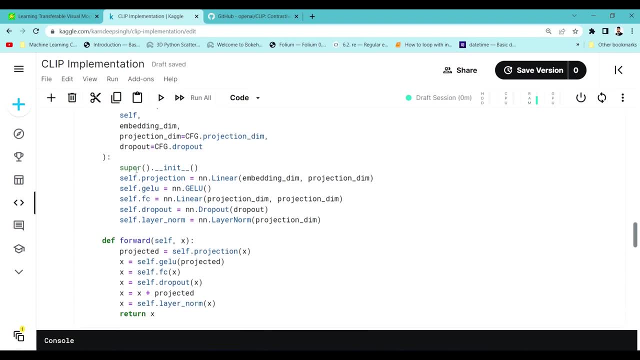 from this particular BERT model, And now this is a projection head that I talked about, where they, where they put, where they pass this output of text encoder and image encoder to this particular projection head to Reduce it to the same dimension space, right to 256 dimension space. 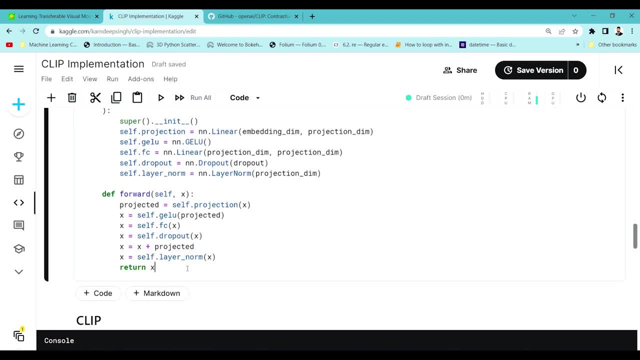 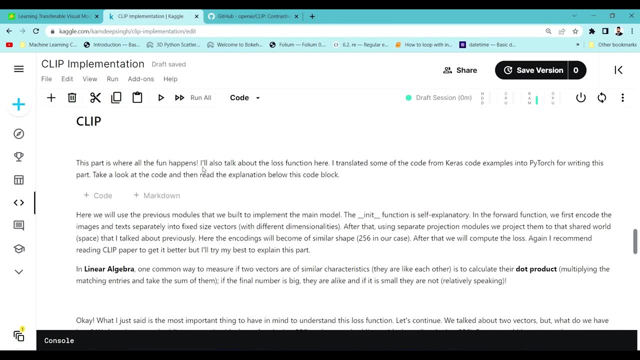 That's what they're doing it, that this is just a normal in network that they're passing it to and will compress that particular text encoder and image encoder output into this particular dimension, right? So once that is done, we just, we just collate this all things: image encoder and text encoder. 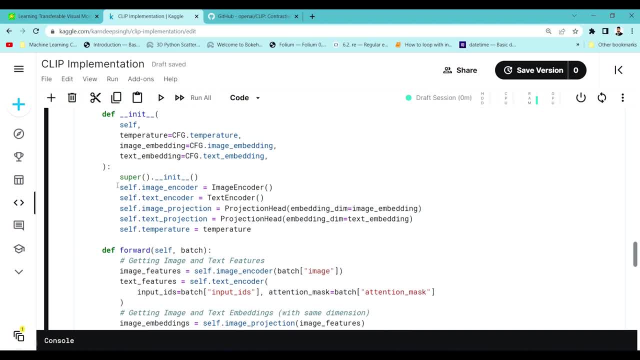 into a single model So you can see, if you see they are loading up this clip model. inside this clip model they are loading up this image encoder, Text encoder, and they're also taking this projection head and they are passing this particular projection head of this image and they are also loading up this text projection. 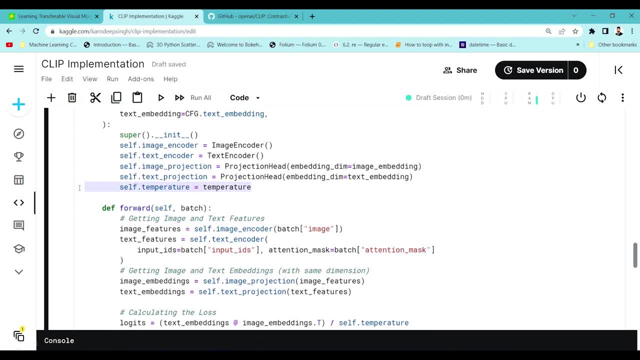 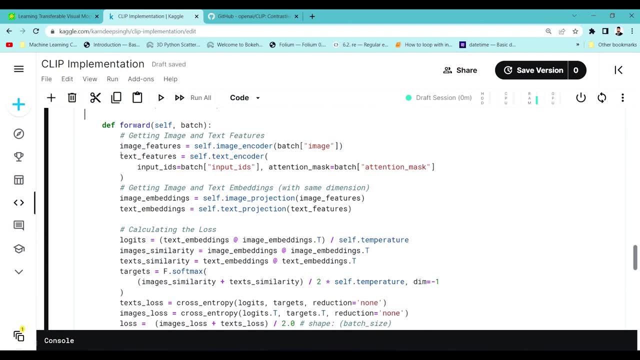 head and the temperature is nothing, but it's just a variation of the like. this is controlling of the projection how you want to how much you want to do it. So if you go into this particular forward output, what it will do? it will take up this. 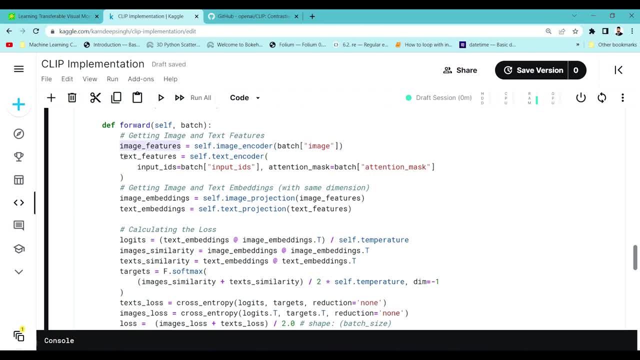 image, It will extract the feature, It will take its respective text and it will pass into a text encoder. right, So you have now. you have image and text features, but these are all of different dimensions, So we want to convert into the same dimension. 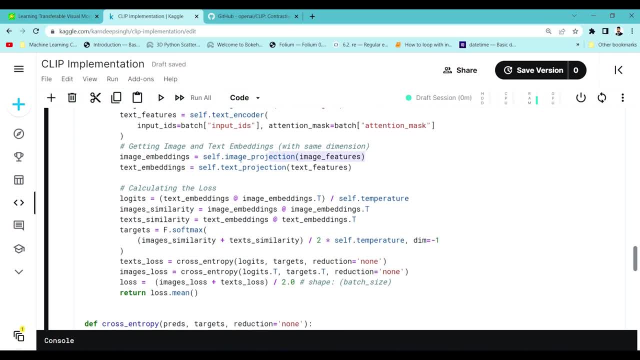 So what they will do is we will pass this image features and text feature to the projection, So this projection will compress that particular image features and the text feature into a similar dimension. So now this particular embedding will have same dimensions. once does, once we have the 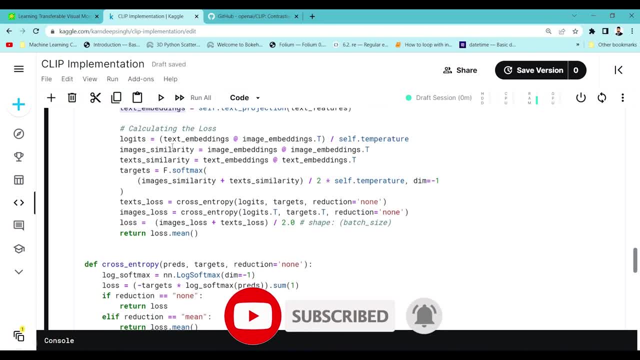 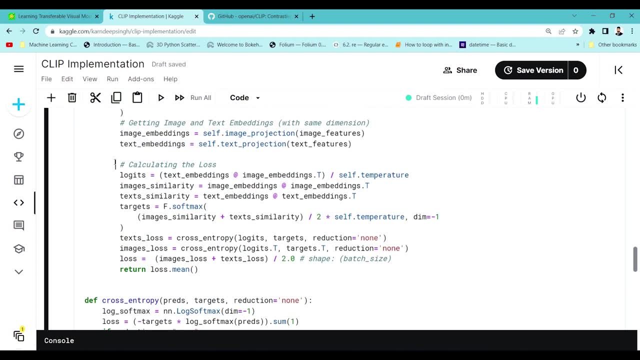 same dimension. So that's why they are doing it now. this is a. this is the calculation part that I've been talking about, about the contrastive loss, So let me go through it. It will be very clear here now. So, once we have this image embeddings and text embeddings, what they're doing is they're trying. 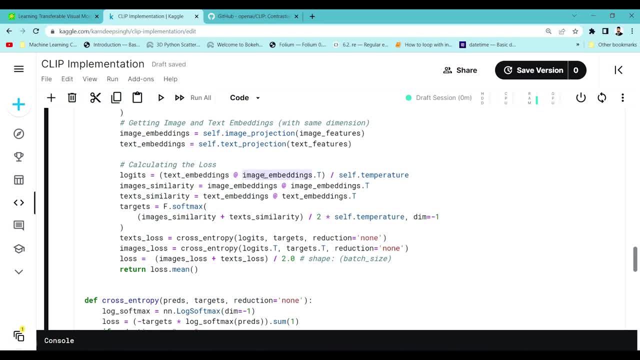 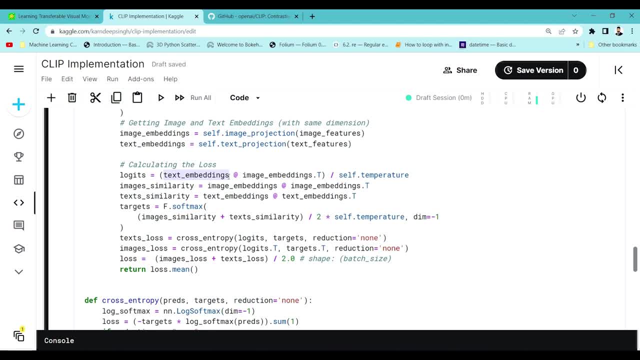 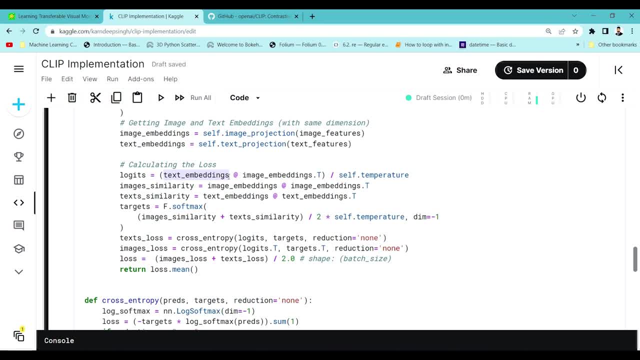 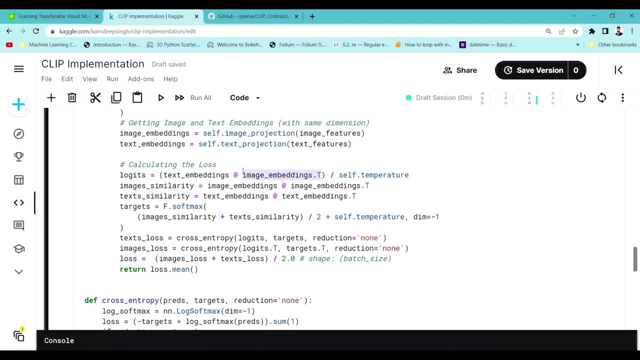 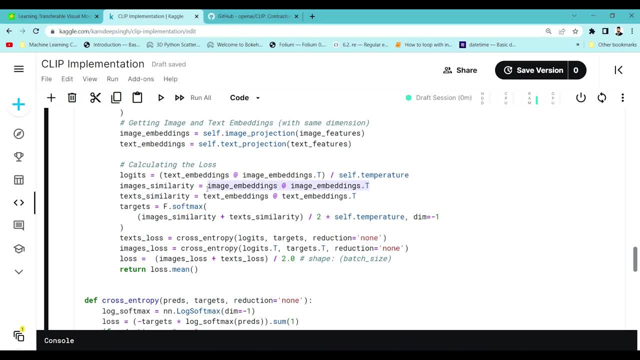 also calculate. we'll also calculate the image embedding and image embedding relationship. so we're also trying to calculate the relationship between the image to its image relationship and image to other image relationship. so obviously the dot word should be very high with respect to the same image right. and similarly we are going to calculate our text embeddings and its other. 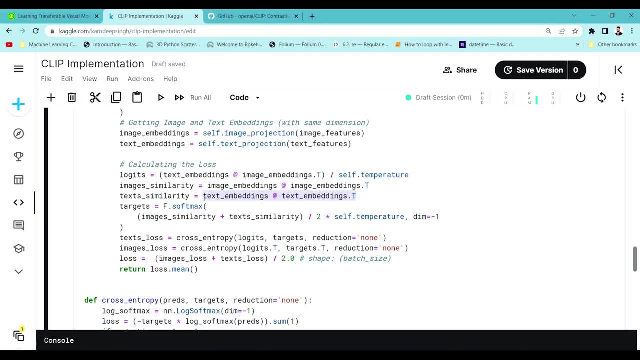 text embeddings, uh, dot product. so we are trying to make, bring the text embeddings closer to each other, uh, by by learning the text embedding from its text embeddings and with other text embeddings. so that's how we are trying to calculate the image similarity and the text similarity. 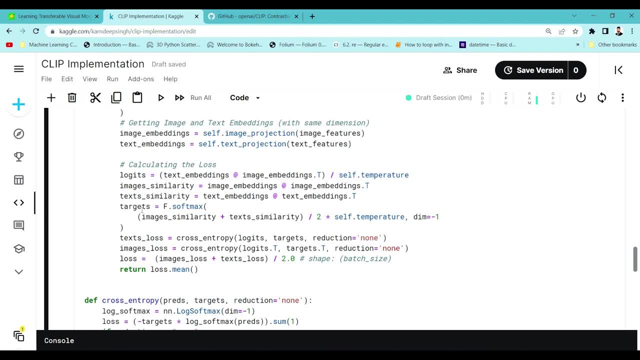 and once we have this, two, these three things, we're going to calculate the targets. right, so this target is nothing but, uh, we are. this is what the target is, right. so targets are nothing but the label that i talked about here. if you see, these are labels, right? so this is what we are trying to calculate, how we are justifying. 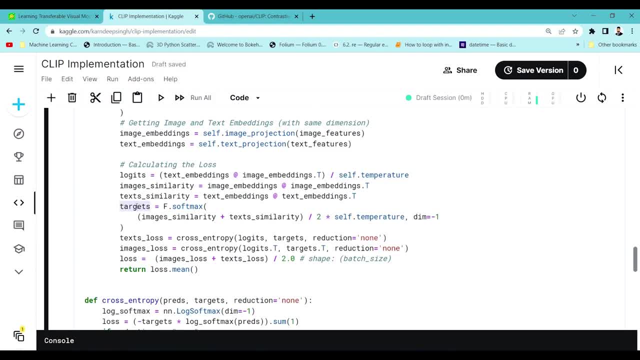 the targets, how we are calculating the targets, how we are making the targets here, because we don't have the targets here. we are trying to meet the targets by own- it's a self-supervised learnings- but we are also trying to calculate these targets by making targets. only we can. 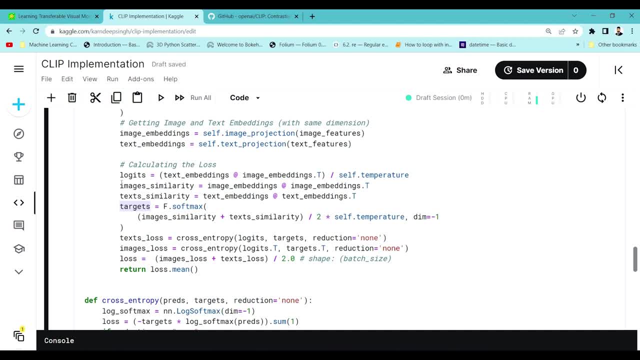 learn right. so, um, the the importance of this image similarity and text similarity was the calculation of this image similarity and text similarity was there because of this, only because, to calculate the targets to label. so in this soft softmax function we are, we are trying to average out this text similarity and image similarity, uh, and we are going to get the target right and once 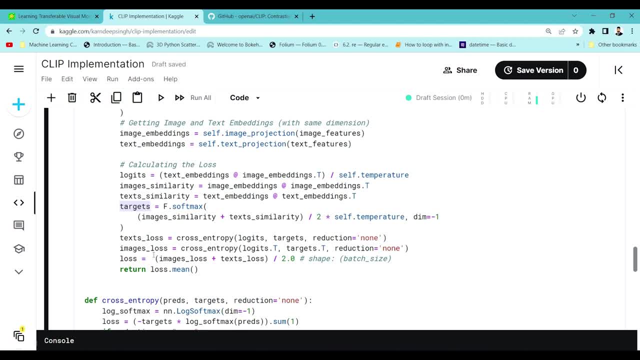 we have this target. that is the label. now we can calculate the text loss and the image loss, and the text loss and image loss are all are very much similar. uh, we are trying to pass the cross entropy. uh, we are trying to use the cross entropy and we are passing the logists that we have calculated. 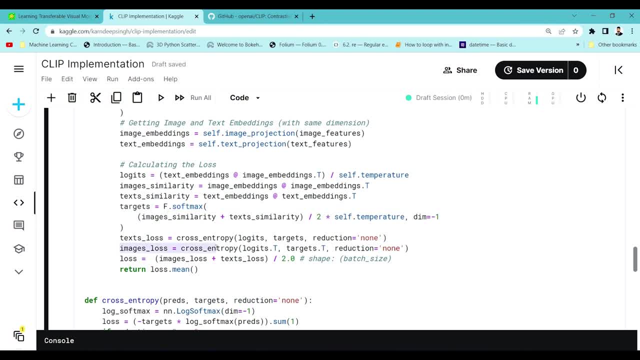 and the targets. these are targets and for the same is similarly for the image loss, we calculate the cross, entropy and logistics and tasks, the targets, and that's how we are going to calculate text loss and image loss and then, finally, we are going to average out this particular losses and then we 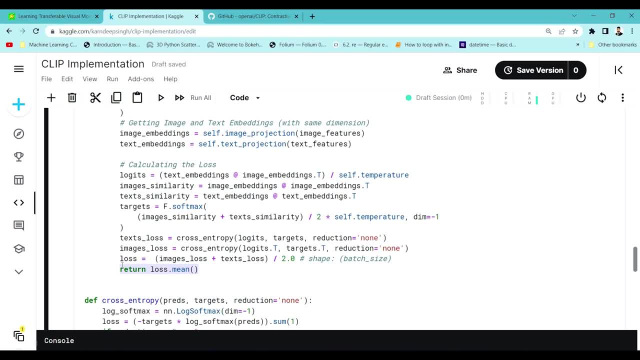 will return the mean of this particular loss. that's how we are trying to do it right, so, uh, so this, this seems to be very, very uh, um, complicated here, but it's very easy. if you just try to explore it out, it's very easy to understand. 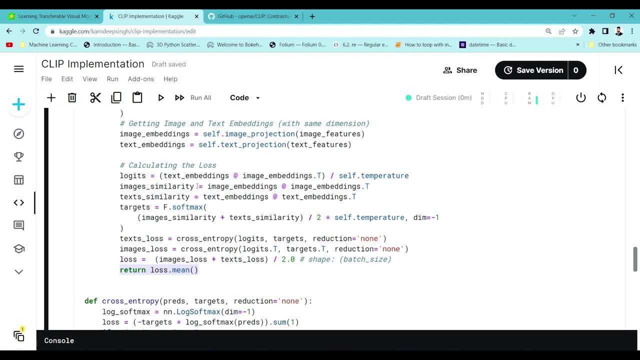 we're just trying to calculate a similarity between the positive samples and as well as the cosine similarity between the other negative samples. so this is what actually it is. it's it's nothing, but it's just taking up the positive samples relationship and negative sample rate. it's like it's like a triplet loss that we're trying to calculate right. so it's just, it's just. 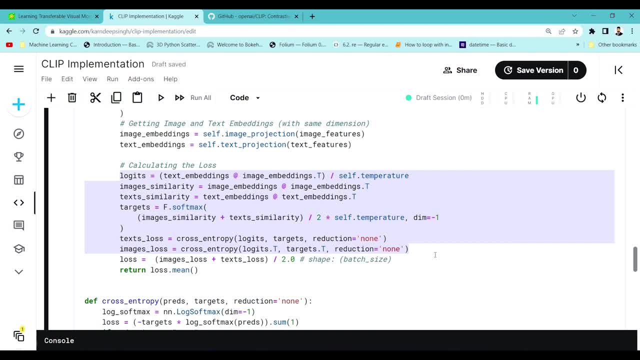 a different way of saying the triplet loss, because in trip let's loss we always have a label, but here we don't have a label. but we are trying to calculate the label by using this image similarity and the text similarity. so that's a different, that's, that's. 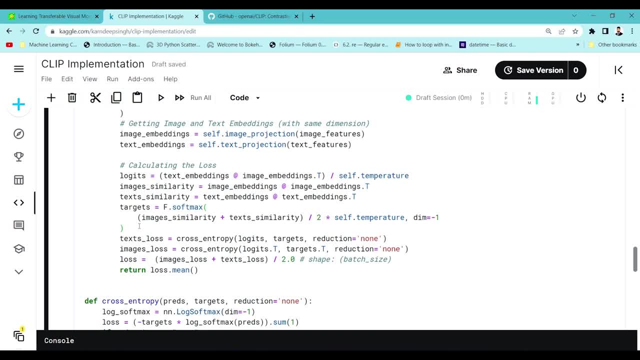 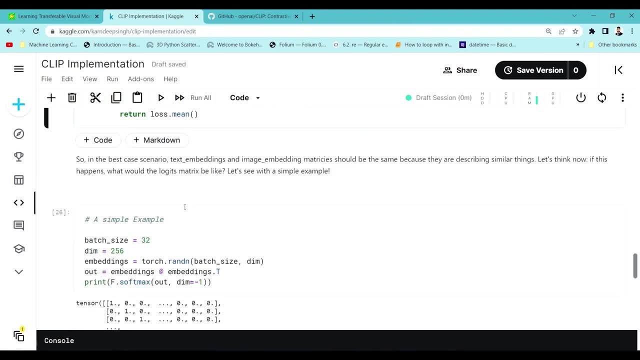 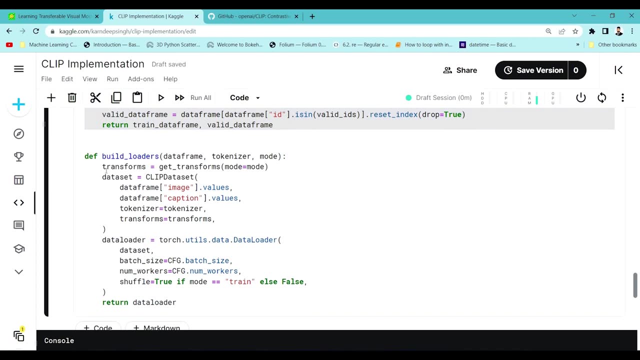 only different. other things are very same, the data is same and that's how we are calculating, right? so that's how, uh, the clip model has been defined. and now, uh, we'll just go to the training part. so here is just, we are dividing our data cycle, train and test, and now we are building up the uh. 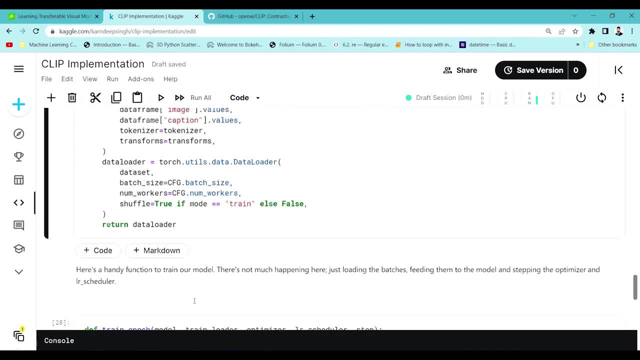 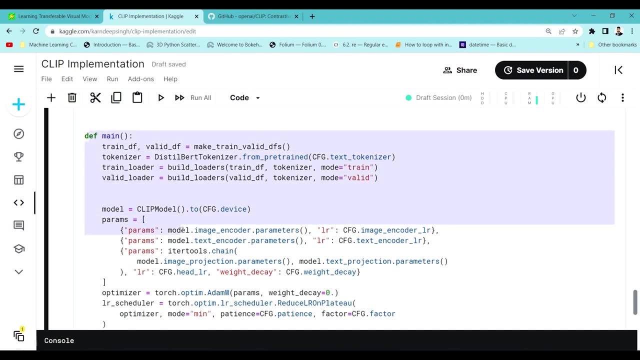 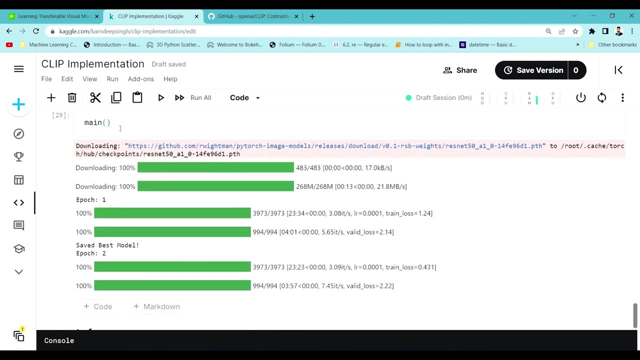 loaders, like we are initiating the loaders, data loaders, and this is a training step and where it's the validation epoch. you can just go through this and this is a main function where we are going to learn about the things and now, uh, we'll train this model by using this, by by running this particular main. 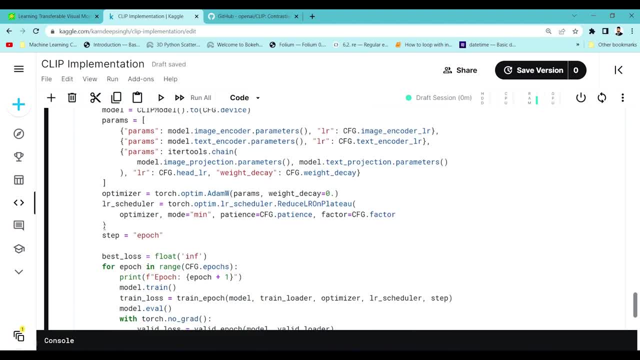 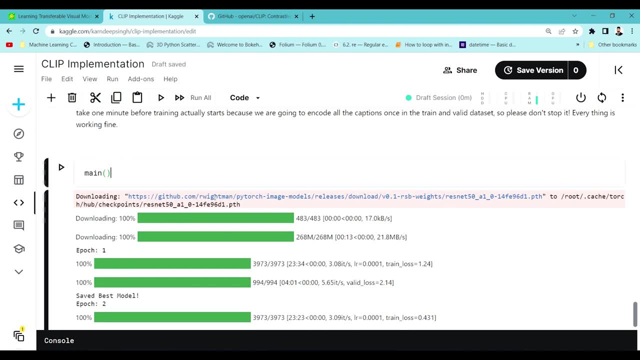 function and once we have this main function, uh, ready, we can just run this particular main function. so before making of this particular video, i ran this particular code. so because it takes a lot of time to train, you can see that it takes a lot of time to train. it takes a lot of time to train. 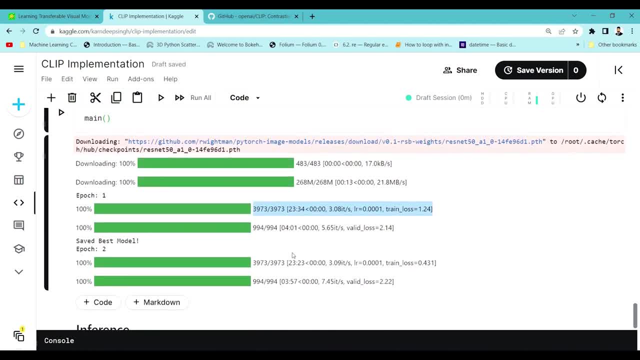 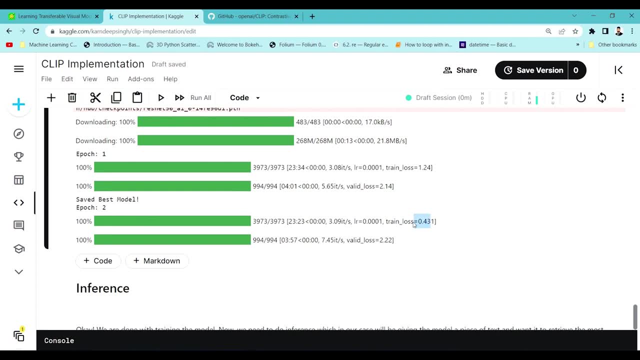 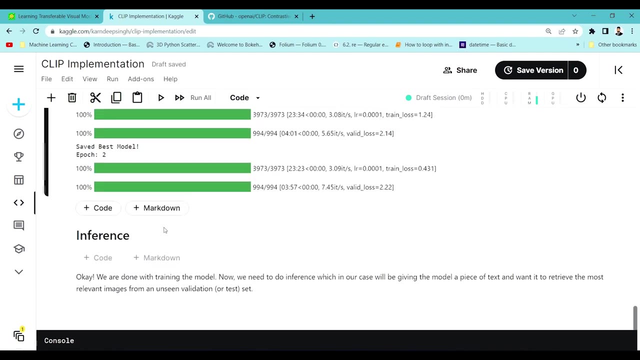 it takes like 23 minutes to 24 minutes for a particular epoch to run. so i trained it already and for this particular demo, and you can see, uh, the loss has converged to 0.431 in just two epochs. so let's, let's just go through the uh like, once the model has been trained. 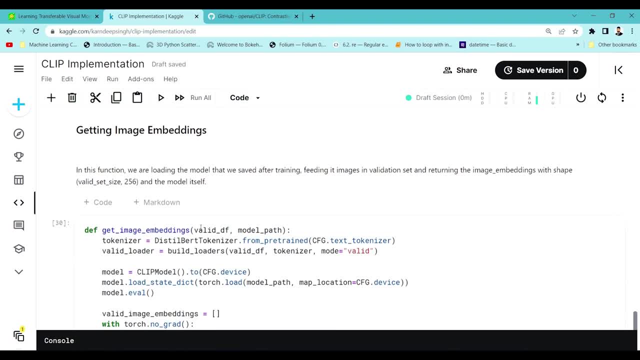 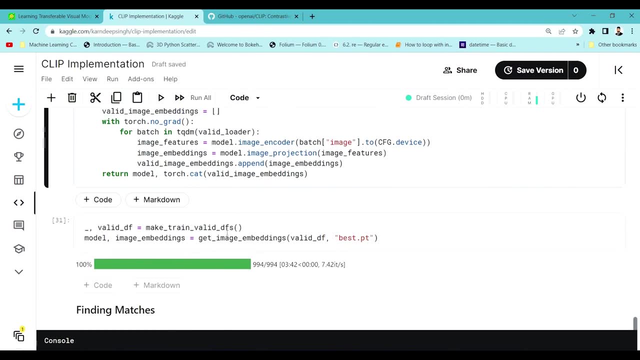 uh, we will just go to the inferencing part, how the things have been done, right. so i will just uh put up this uh function which will take up this embeddings of the particular image is and the text, and it will generate uh embedding for us. so what this uh particular function will? 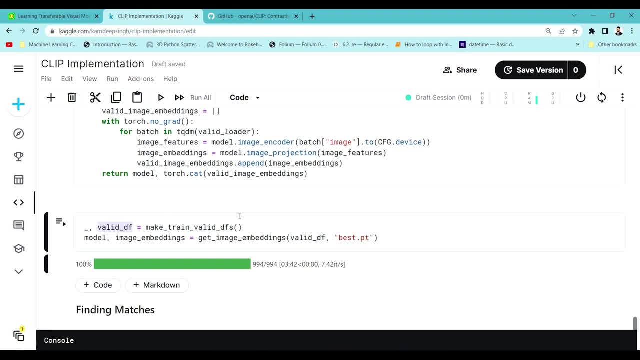 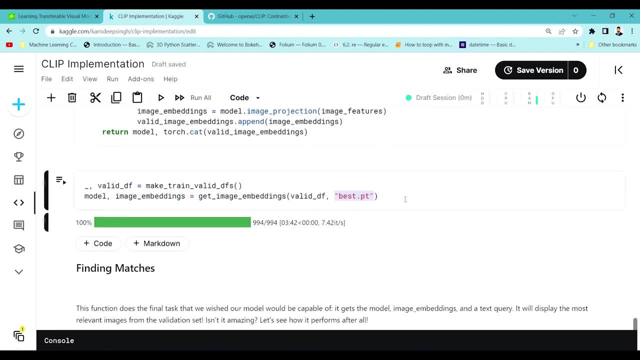 do? it will take the data set- uh, whatever data set, validation data set- and it will take up the uh best model that has been trained and the trade here, the model that we have trained here. it will take these two paths and it will generate an embedding for the images and it will also. 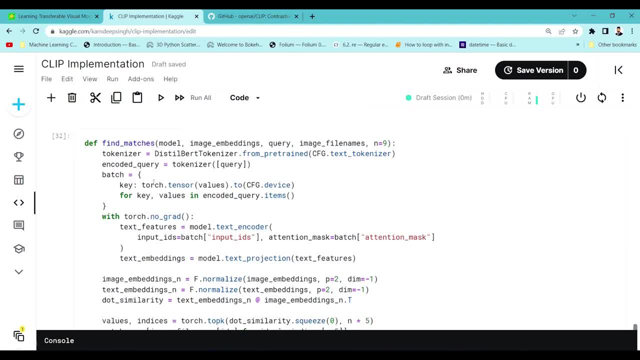 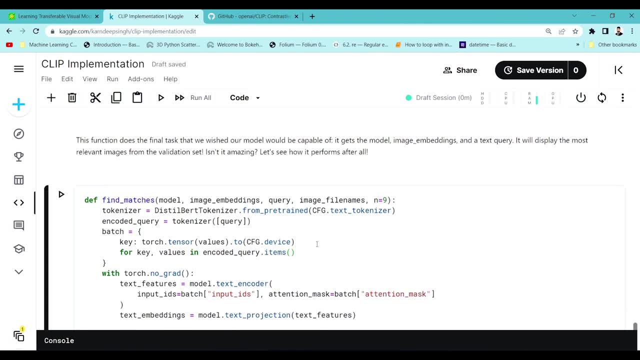 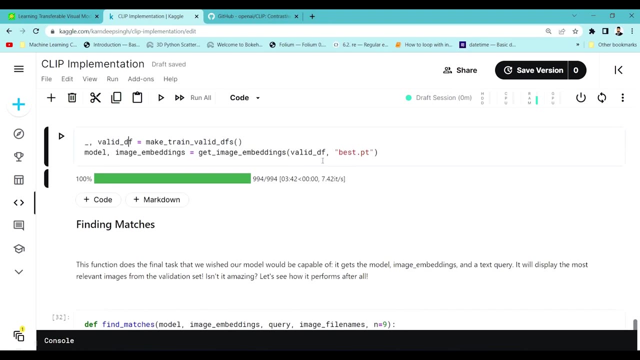 return them on. so once we run this particular code uh, we can use uh, our, our particular uh embeddings to generate uh, uh to find the images right. so this particular function help us to evaluate the model. so once we have loaded the embeddings and calculated the uh, loaded the model. 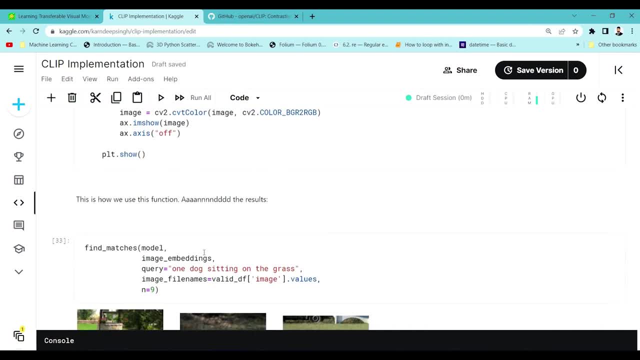 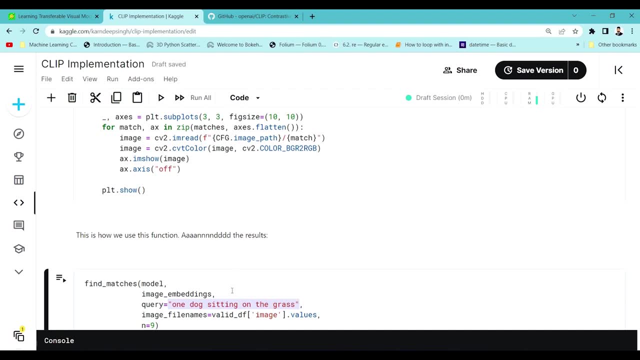 in here we can calculate actual matches, so we will just pass these images. we'll just pass this text to the model and it will try to get the right images for us which are associated with this particular text. so what is actually it is doing is if we are going to pass this particular 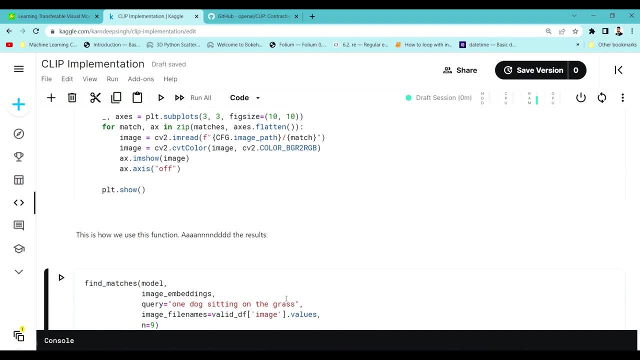 text, like one dog sitting on the grass. so it will just try to find the uh image which is very sim, which is very close to this particular uh with this particular text, or which has this similar meaning uh which has similar meaning to this particular text. so it will just try to find out the. 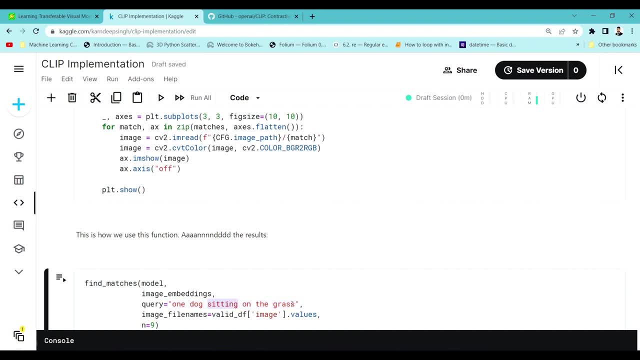 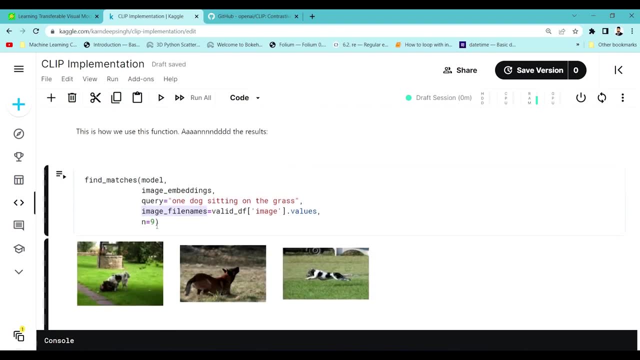 images: uh, from the from the data frame or from the from the data set to extract the images of the similar meaning. so let's pass this and you can see it is. uh, it has quietly extracted the things out from the images. you can see the dog is sitting on. 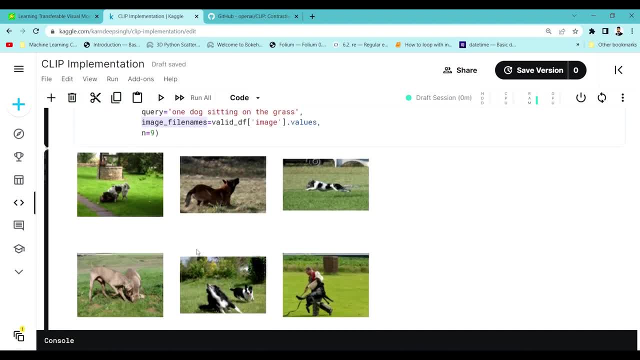 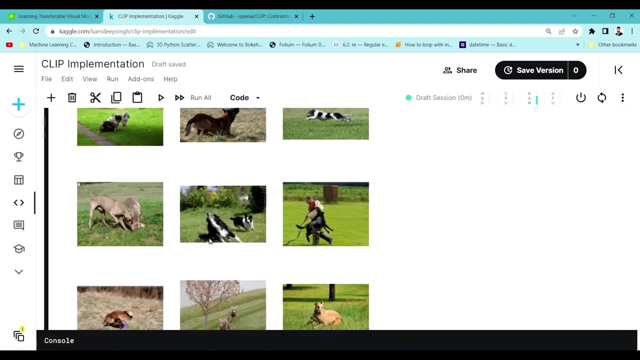 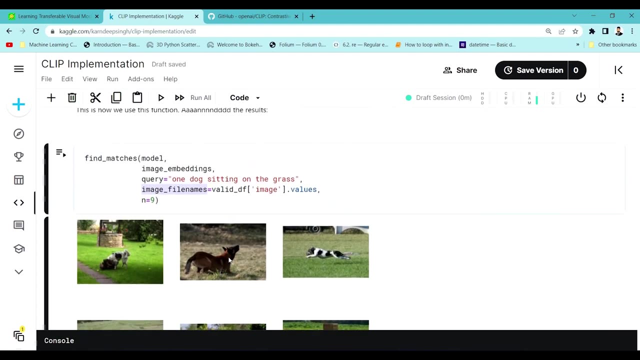 the grass right, the dogs- one dog- uh, it's not a, it's a dog. so these are the things, how it is being doing. so it is actually finding a relationship between the text and the images and you see how it, how it is beautifully- and understanding the context of the image and the 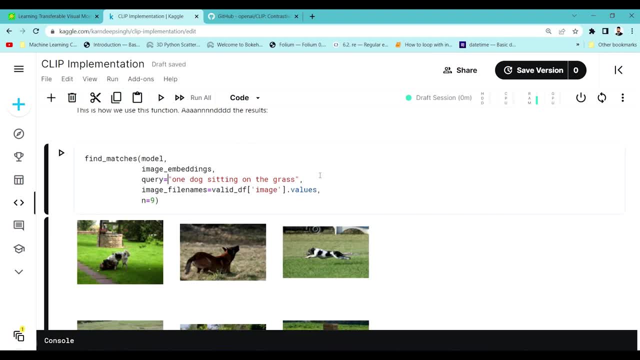 uh, uh on the and the text right so you can use it. you can use the embeddings of this text and the image for your n number of cases. so this, this is one part of you know the user that you can build up um. so once you have this model, drain.